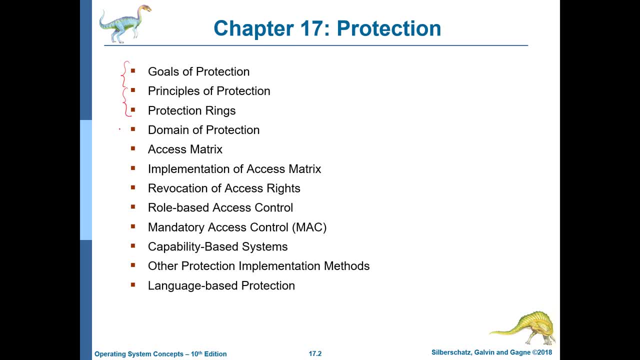 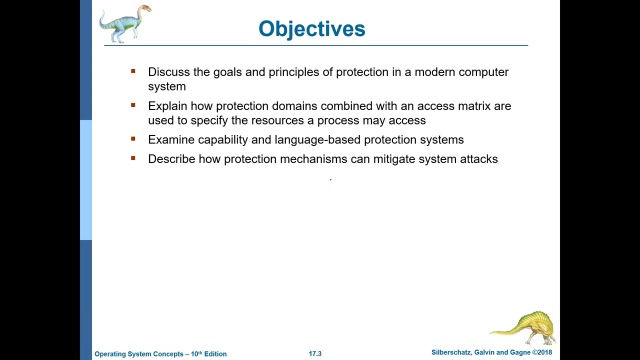 Then we will talk about two main mechanisms. The first is access matrix-based mechanisms and the second are capability-based mechanisms for protection- And finally conclude with a few advanced aspects of protection: operating system protection. So the objectives of this chapter are as follows: The first is to discuss the goals and principles of protection in a modern computer system. 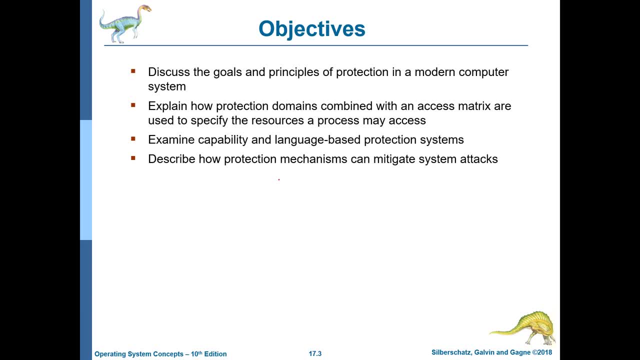 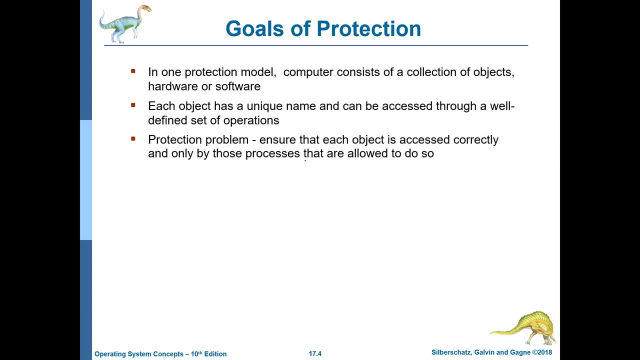 Then discuss access matrix And finally describe how protection mechanisms mitigate the risk of attacks. So what is the goal of protection? Well, in a protection model, we would like to protect objects, where object can either be hardware or a software object, from malicious attacks. 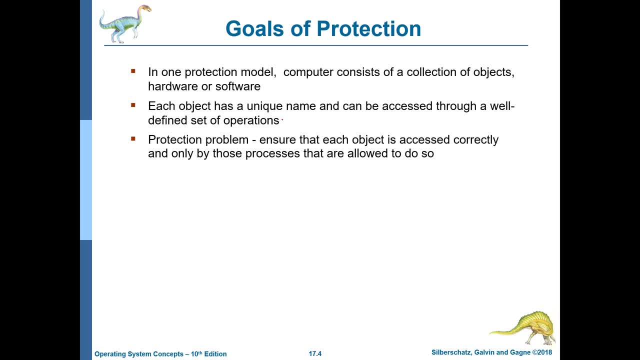 So each object is identified by a unique name and it can be accessed by a well-defined set of operations. So the main aim over here is to ensure that each of these operations are protected, in the sense that they are accessed correctly, the way they are intended to be accessed, and they are also accessed by those processes that are allowed to do so. 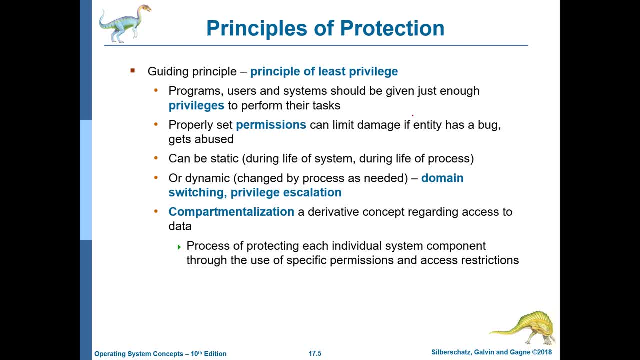 So what is the main principle of protection? Well, it is the principle of least privilege. So this means that, be it any entity, a program, a user, a system doesn't matter, It is given just Enough privileges for it to perform its task, and not more than that. 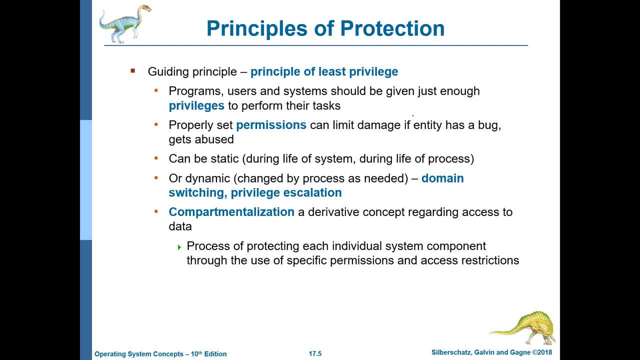 So, of course, if there is an attack, in the sense if there is a bug or if there is an external attack, if the permissions and the protections are set correctly, they will limit the extent of the damage. They are typically static, in the sense during the lifetime of a system or during the lifetime of a session. they remain the same. 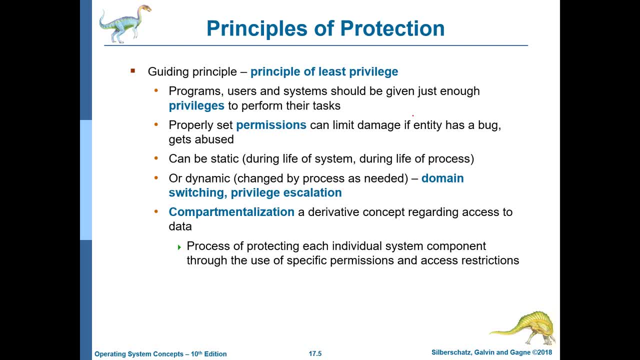 But they can also be dynamic, in the sense they can change if needed. So, for example, let's say that we want to switch a domain go from a user mode to administrator mode. then we can escalate the privileges, we can increase what we have for some time. 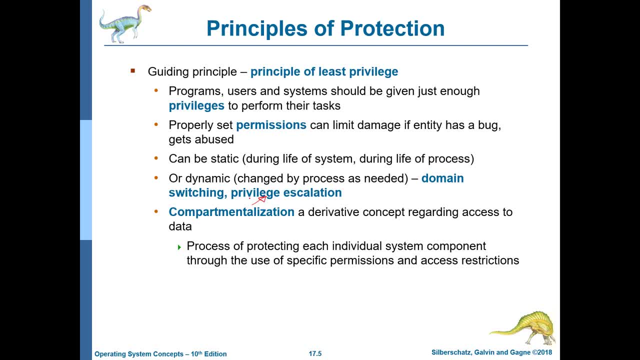 Then there is something else, which is a related concept, known as compartmentalization. So this is a derivative concept. This is regarding access to data. So this is basically the process of protecting each individual component. So we take every individual component of an operating system. 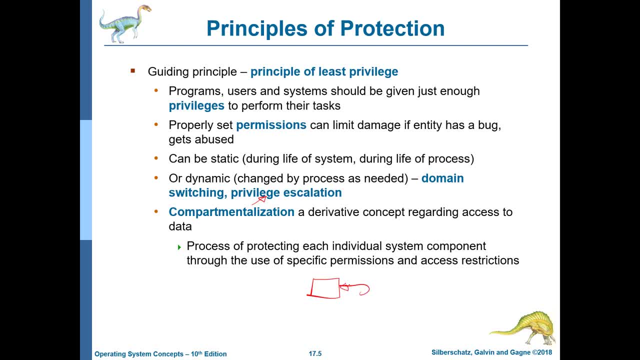 And then we provide very specific permissions and access restrictions. So in general, this can be. this is a generic mechanism, so this can be done at the level of individual components, like files, for example, Or it can be done at a larger unit, like directories, for example. 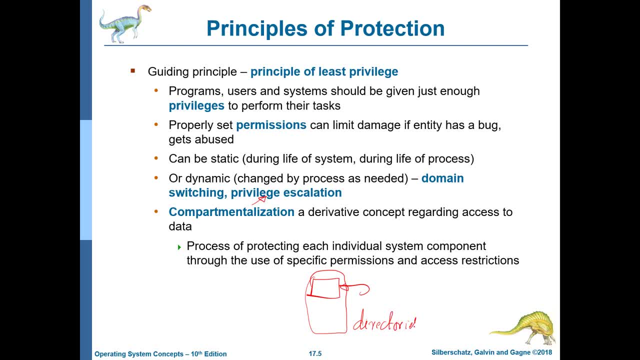 So there we can, you know in detail, say who is allowed to do what, who is not allowed to do what, so a full list of do's and don'ts. So of course this can be a pretty cumbersome exercise. 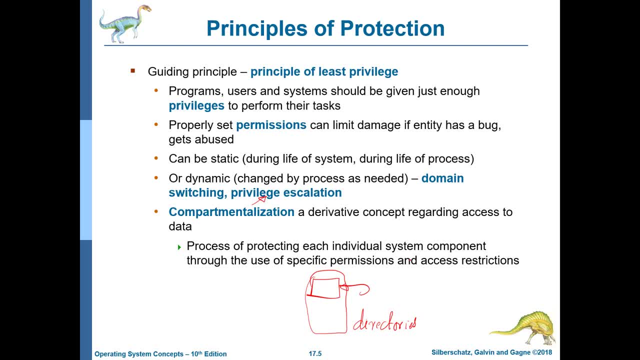 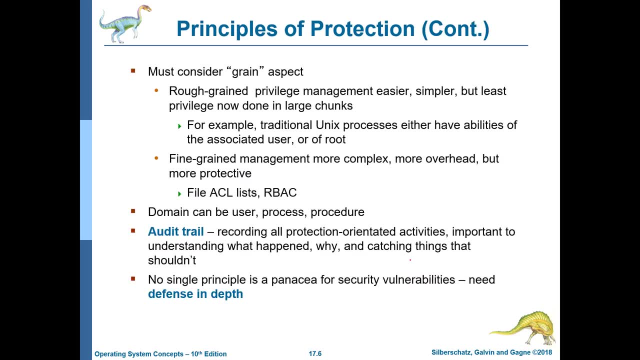 Particularly. if there is a problem, then we can do it. we have a lot of users, but then that is said and done. in many commercial systems this level of protection is often required. So we should look at whether we are looking at like a rough grained privilege management. 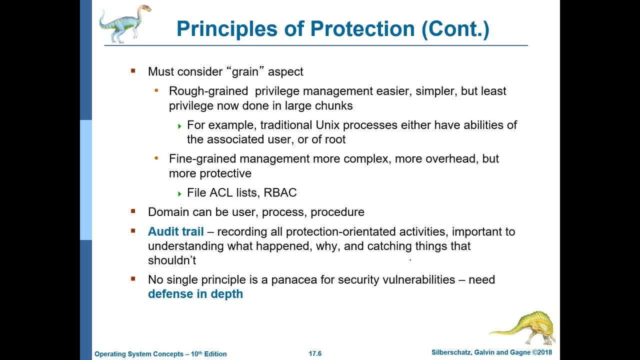 For example, if you look at UNIX systems and UNIX processes. so we have already discussed the notion of the user, the group and all. but this is fairly coarse grained in the sense that you do not have to specify a lot. you just set the user ID and the group ID of a. 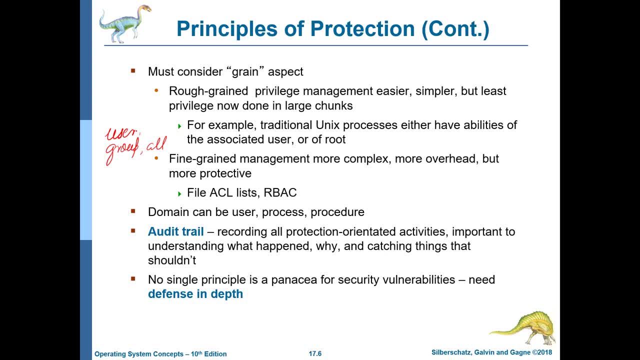 file and the rest. all is taken care of and maybe some processes can be initiated by the user, some by the root. So root or the super user is a special user who has some more access to the resources of the operating system as opposed to a regular user. 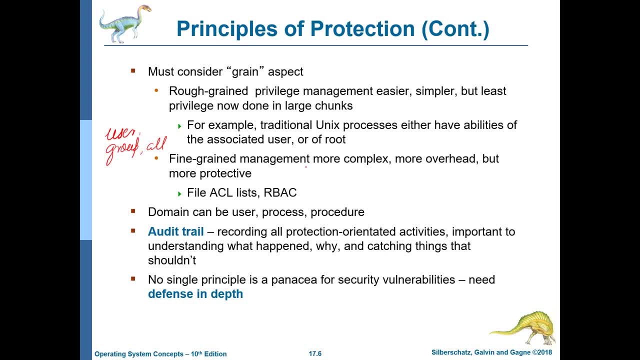 Fine grained management can be far more complex and far more cumbersome from the point of view of system administrators. And even if you are a system administrator, you are not going to be able to do that, So you have to be able to do that. 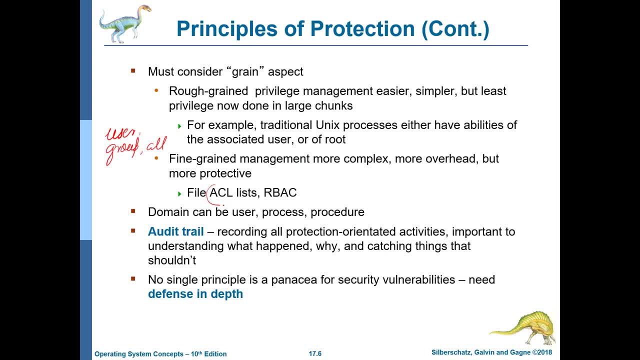 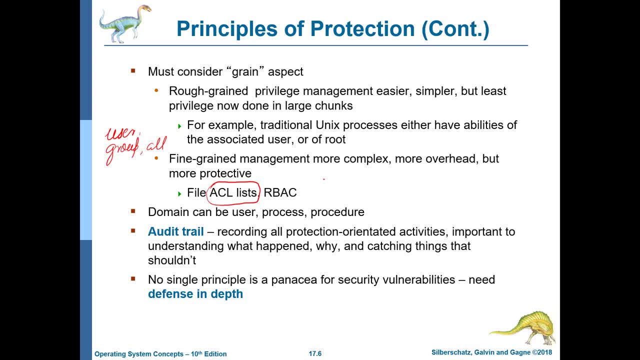 So we could have that, and then this could be specified in detail if there is a need, that is. The other mechanism is RBAC, which is also called role-based access control. So in role-based access control, what happens is that the access is not given at the level. 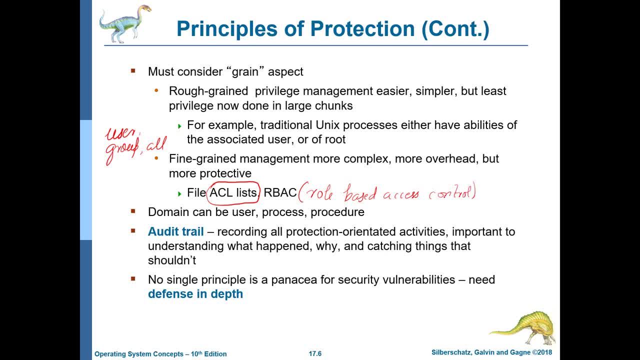 of individual users but is given based on the role in the company, Like, for example, managers can have a certain level of access control, senior managers can have a certain level of access control, vice president and so on. Furthermore, we can make domains, in the sense we can group users into sets and each set 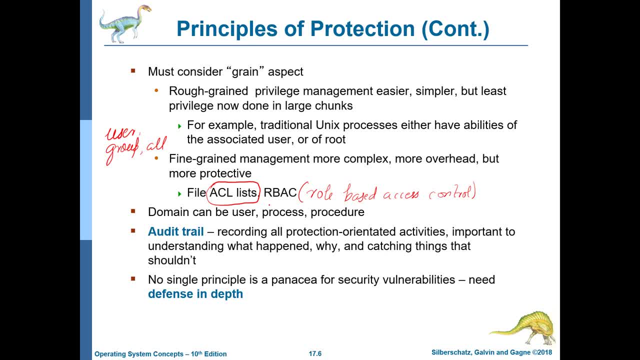 will have a certain level of permission and, of course, whatever is done, regardless of whoever is doing it, needs to be audited such that later on it can be analyzed in great depth, which means anytime we change the protection of any file, particularly that needs to be. 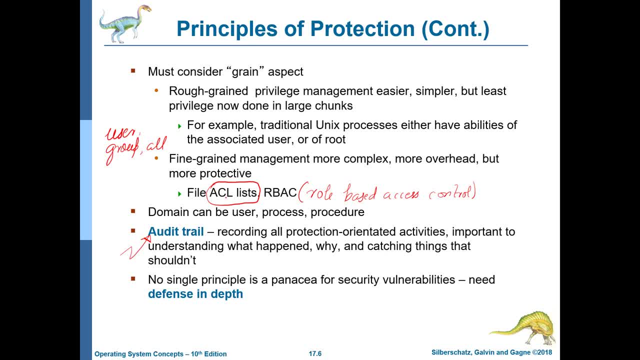 recorded and audited such that we can catch things. and nowadays, of course, there are many machine learning based tools that can automatically analyze such audit trails and figure out if something is amiss. So if something is amiss, then immediately maybe the system administrator can be told. 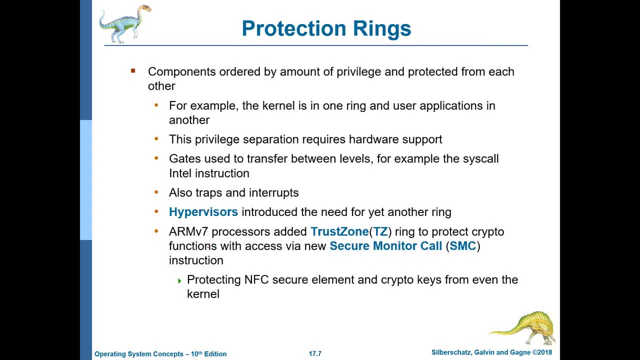 that look, something is going wrong. So one of the key ideas in protection is the notion of a protection ring. So protection ring as such is a hardware concept. So what we do is that let us say we have rings of this type like ring 0, ring 1, ring. 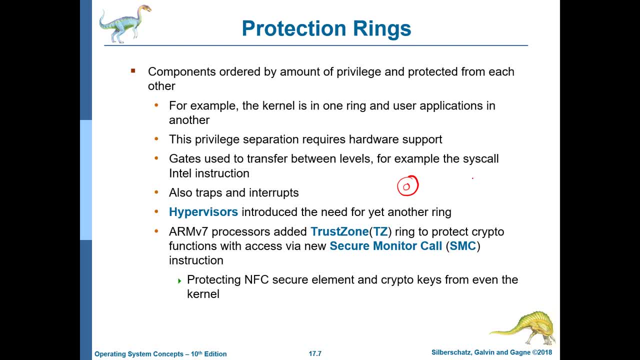 2 and ring 3.. So a ring is nothing but a register. So a ring is nothing but a hardware register. So if there are four rings, it is a two bit hardware register. Typically what happens is if we do not have anything. so what is the hypervisor? I will 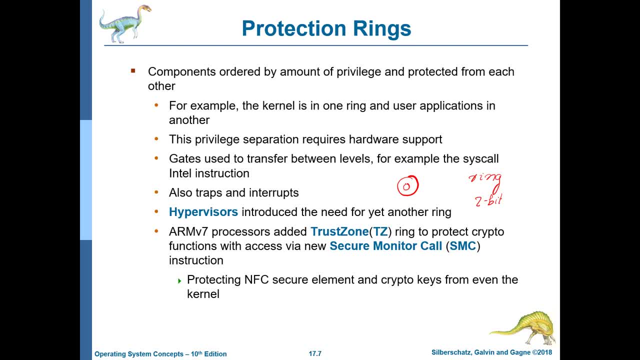 tell you later. but let us say that if we just have the operating system and we have a user application, then what can happen is that the operating system, let us say, can run in ring 0, which means that it will have accesses to all the devices and all the files. 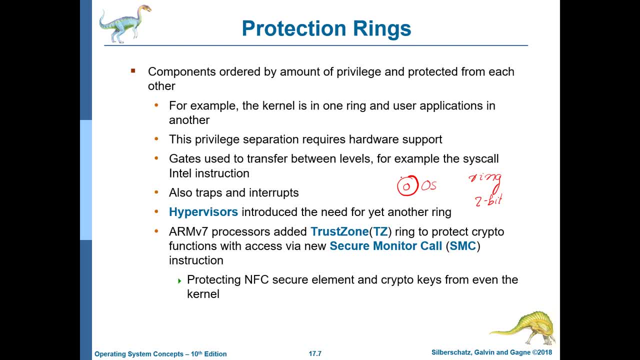 So anything running on ring 0 has the access, has the access to the maximum amount of hardware, Then of course we can. we will have ring 1,, ring 2,, ring 3,, ring 4,, ring 5,, ring 6, ring. 6, ring 7, ring 8,, ring 9,, ring 10,, ring 11,, ring 12,, ring 12,, ring 13,. ring 13,, ring 14,, ring 13,, ring 14,, ring 15,, ring 15.. 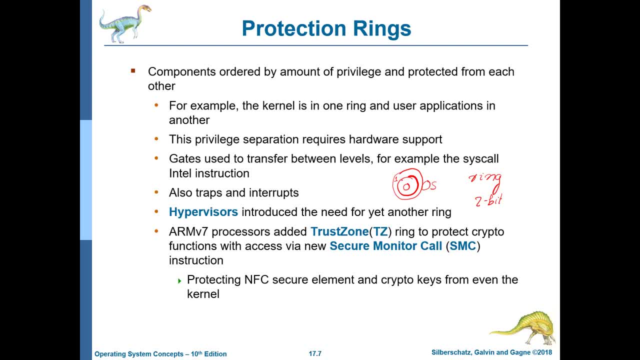 So this is again another hardware concept, So it may be here in ring 0, you can access the BIOS. in ring 1 you cannot. Similarly, ring 2 will provide less and ring 3 will provide even less. So let us say that applications can run in ring 3, where they will not have access to. 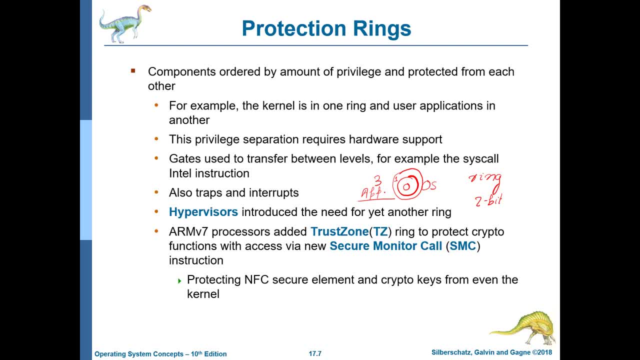 a lot of instructions and a lot of hardware resources as well. all right, So of course it is possible to transfer between levels. for example, when an application makes a system call, Then the control automatically gets transferred to ring level 0,, which is the ring of the operating. 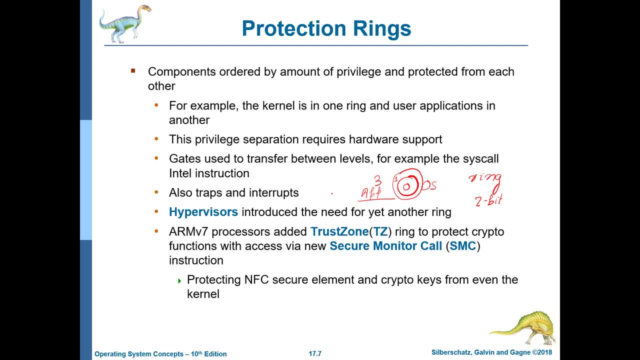 system all right, And traps and interrupts can do the same thing. Modern systems also have a specialized program called a hypervisor. So in this case the hypervisor is some is a program that will run on ring 0. And the operating systems typically run in ring 1 or ring 2.. 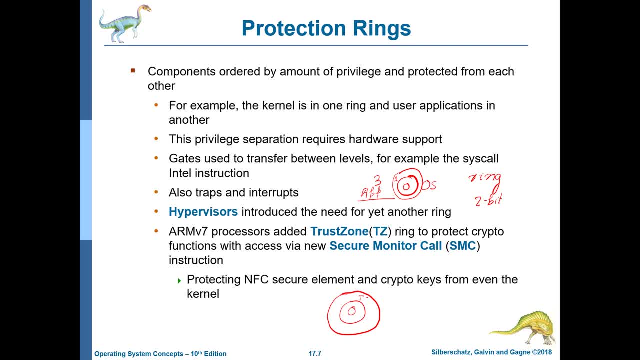 So the hypervisor is like a super OS In the sense you would have typically seen programs running on ring 1 or ring 2.. You would have typically seen programs such as virtual box or VMware, which allow you to run another operating system as a regular application right. 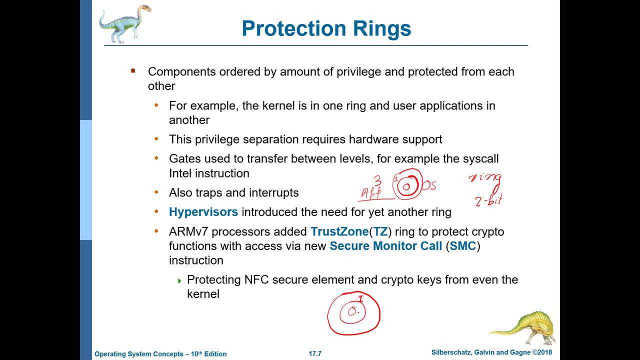 So what normally happens in modern systems is that on the CPU we have a very thin operating system that is running. it is called the hypervisor, And the hypervisor furthermore runs a regular commercial operating system or a regular operating system like Windows and Linux on top of it. 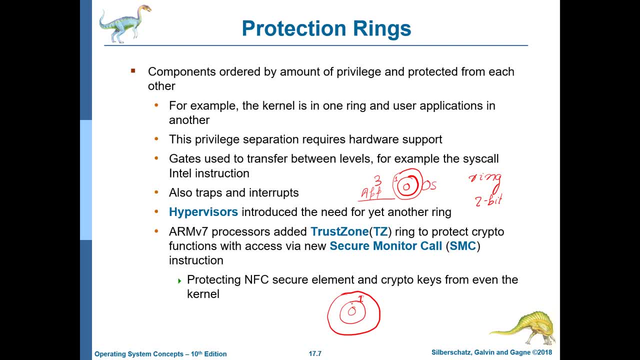 All right. So that is the key broad idea over here- that we run other operating systems on top of it. So these operating systems will run like applications and, of course, their powers with regards to hardware will be limited, as opposed to the hypervisor. 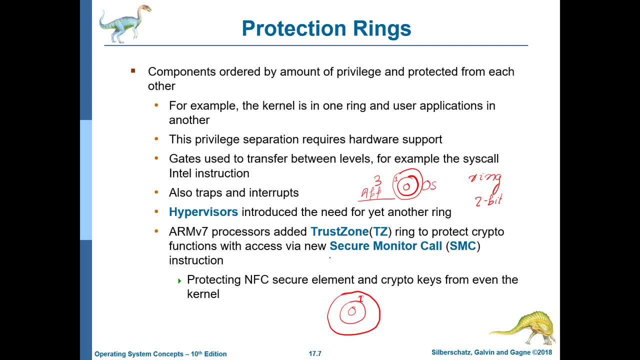 And the hypervisor will be discussed in a subsequent chapter. Furthermore, we can have dedicated secure hardware like ARM Trust Zone or Intel SGX which can run on a regular operating system All right. So that is the key broad idea over here, that we run other operating systems on top of it. 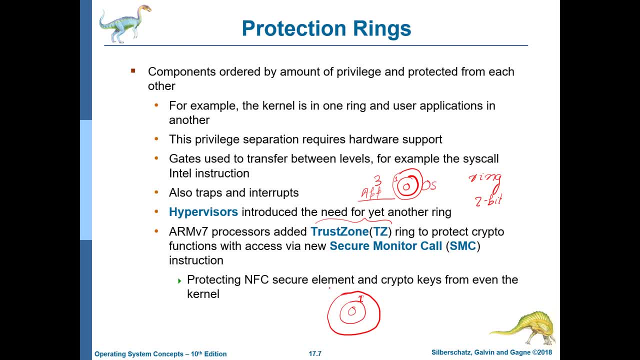 So we can do secure actions, particularly in systems where we do not trust the kernel. For example, Intel SGX can be used to securely load a program and execute it and the kernel will not be able to tamper with it, And furthermore, it is possible to send evidence to a third party server that the kernel indeed 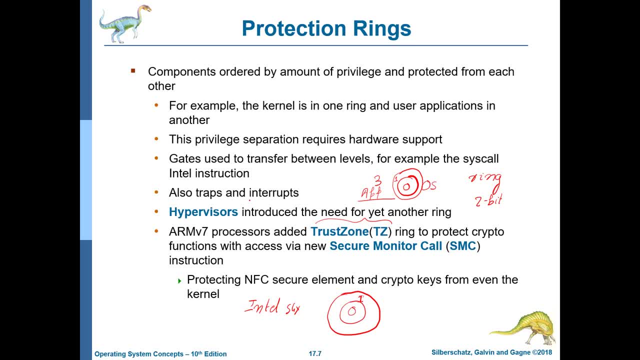 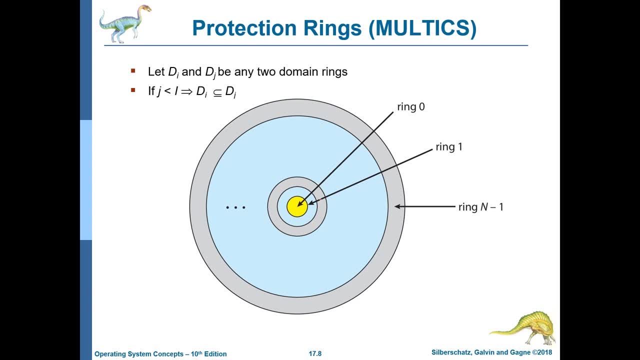 has not tampered with the execution, So that is also possible with secure hardware. So, as I said, the idea of protection rings is like this: That we have. we can conceptually arrange them in this manner: The ring 0 runs with the highest privilege and gradually applications run at the outermost. 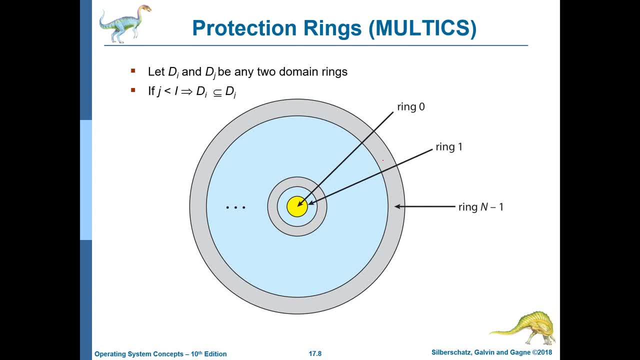 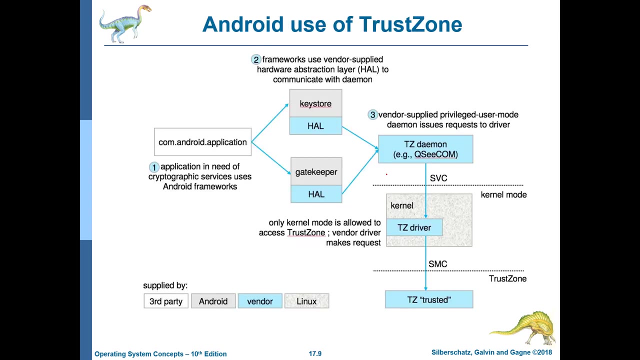 rings, which means that they have the least amount of privilege And, needless to say, the hierarchy is inclusive, which means that ring i, or let us say maybe the ring 5, can do whatever ring 6 can, but ring 6 cannot do everything that ring 5 can. 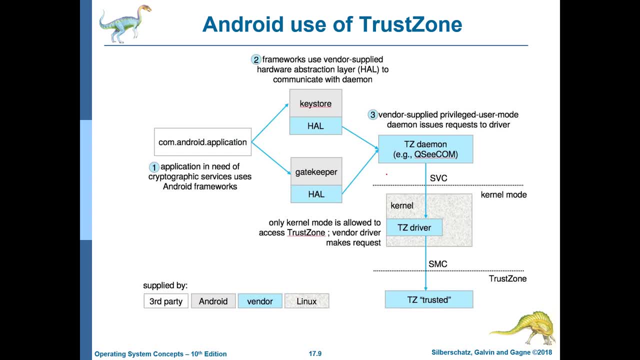 So Android does use ARM trust zone. So ARM trust zone is a mode of execution and also some additional hardware where applications can run securely in the sense that what they are doing will not be visible to other processes, including the kernel. So any application that is in need of cryptographic services will use the COM Android application. 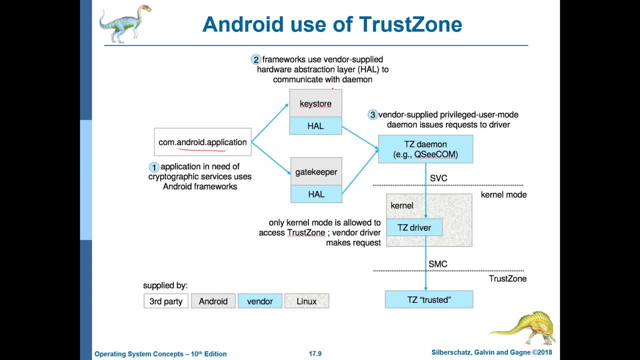 Frameworks use vendor supplied hardware abstraction layer to communicate with a daemon, And so the hardware abstraction layer basically allows you to abstract the hardware such that you can communicate with the trust zone daemon. So then this is vendor supplied, in the sense that whoever is supplying the chip that provides 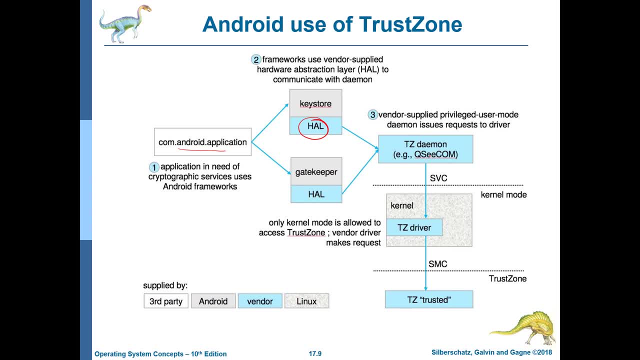 a privileged user mode daemon. So this issues a request to the trust zone driver via the kernel and then the kernel basically sets up what is called a trust zone. So this is basically a trust zone secure area or a secure region where the program 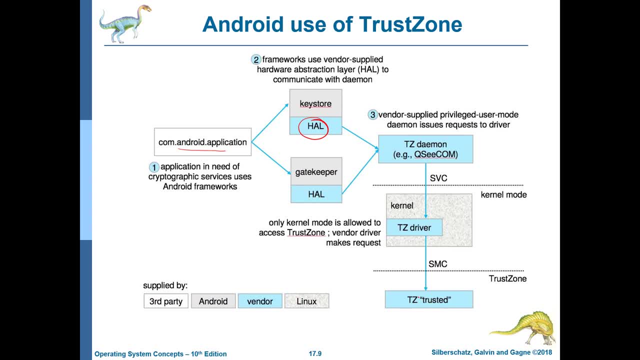 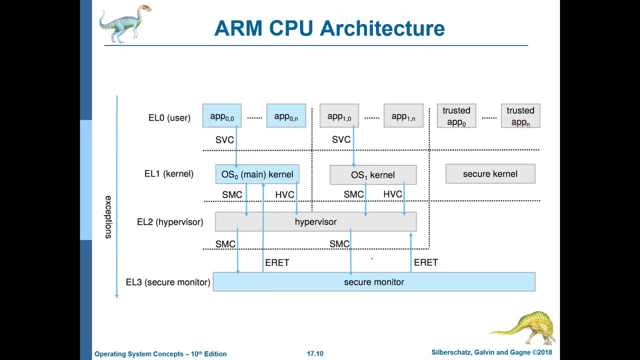 can execute on a secure process and with and within the trust zone mode, the program can execute securely. So in this case it is guaranteed that it can perform cryptographic operations without other processes, and even the kernel, for that matter. seeing it So, the ARM CPU architecture is like this: 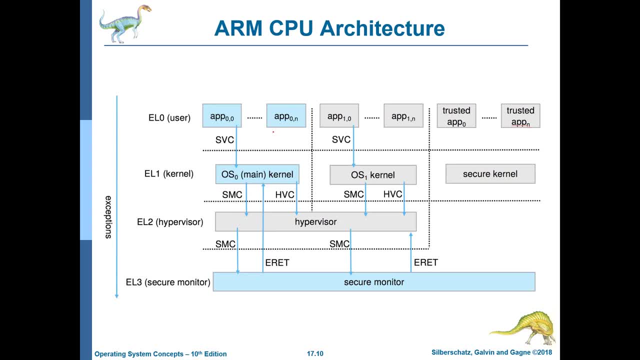 So we have applications, applications at the user level. they trap to the kernel and if, let us say, hypervisor is running which, as I said, is like a very thin layer of code whose job is to mainly run different OS kernels, so a modern hypervisor can run different OS kernels in parallel. 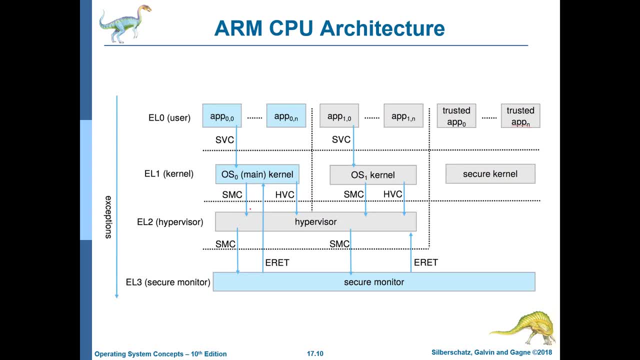 right. So how do they exactly run? well, we will see that in a later chapter. And then, of course, there will be a security monitor that will monitor all the activities of the hypervisors and the kernel. in addition, it is also possible to run a set of trusted 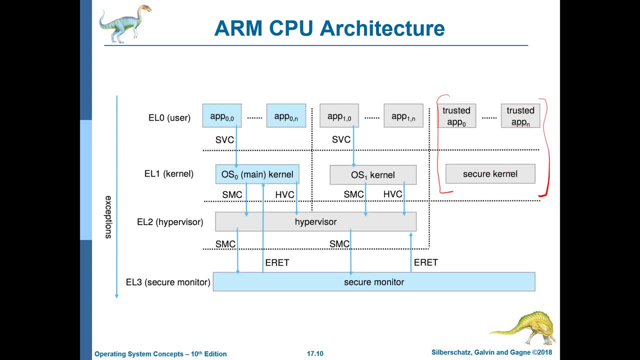 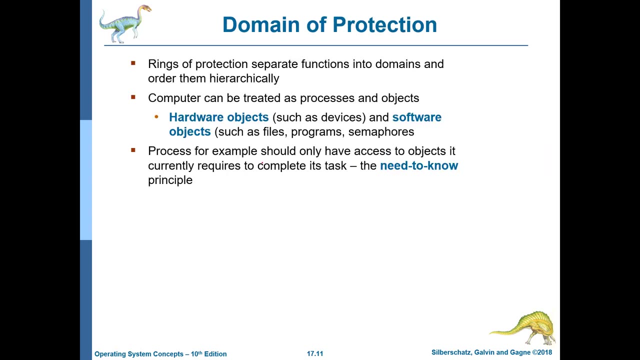 applications in the secure mode, in the ARM trust zone mode And in this process. what will happen is that whatever the process is doing will not be visible and other processes also will not be able to tamper with the state of the secure process. So, coming to the domain of protection, our main aim is that any computer can be treated. 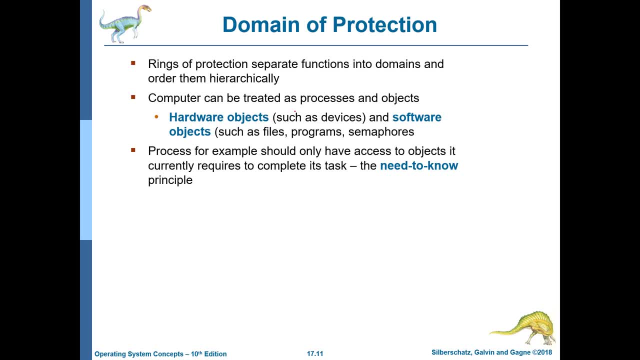 as a set of processes and objects, where the hardware objects are the devices and the software objects are the files, programs, pipes and, of course, etcetera. Any process from the principle of least privilege should have access to only those objects that 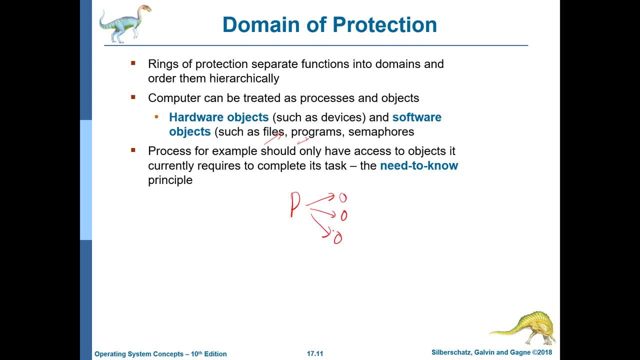 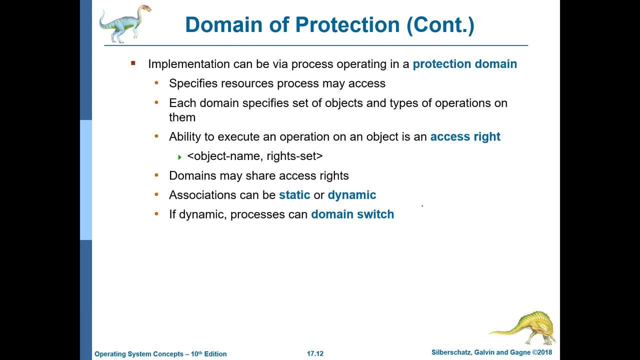 it needs to access or needs to know about it should not have more access than what is genuinely required. So, as we have discussed before, any kind of a protection Domain will basically have to specify all the resources that a process may access. 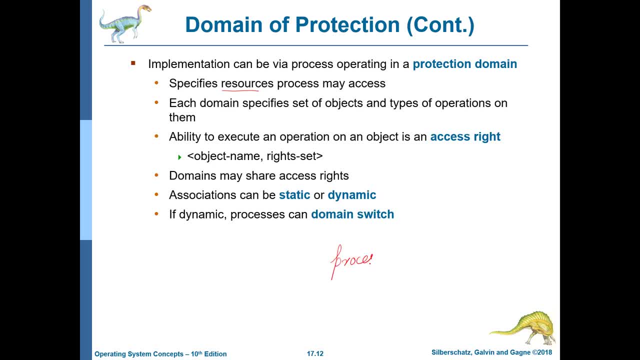 These can be hardware resources or these could be software resources. So, given a process, we either can have hardware resources or we could have software resources. Furthermore, the ability to execute an operation on an object is again an access right. So for given the object, we could have a set of access rights along with it. 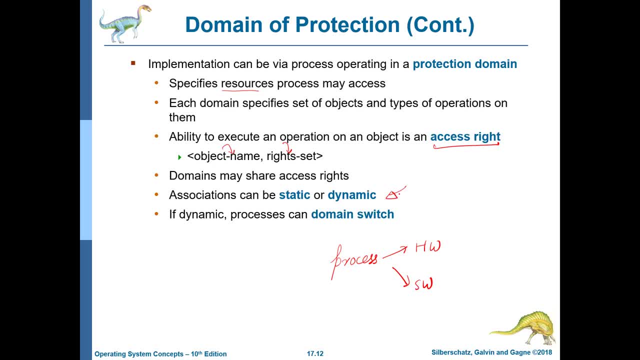 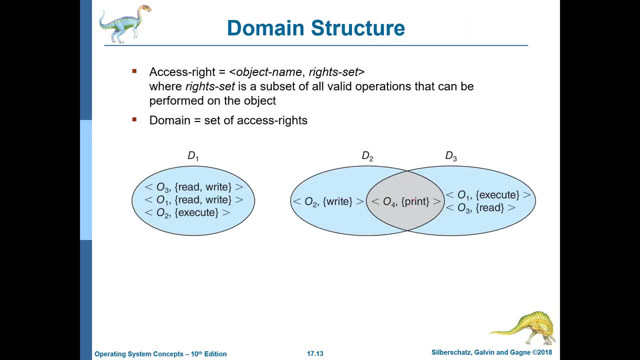 And, furthermore, domains may share access rights which can be either conferred to the object statically or dynamically. This is something that we have discussed. So the access right as such is an object name and set of rights, a right set. So, as we can see, let us say, one domain gives read, write access to object 3, read, write. 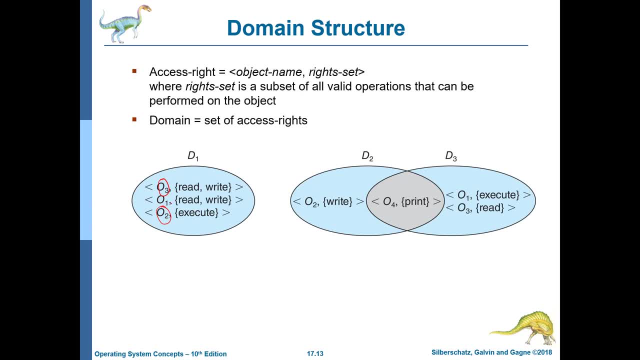 to object 1, and executes access to object 2.. Similarly, two domains can also have an intersection where the same right is kind of shared between two domains. This means that any user that is part of any of the different domains can have a unique. 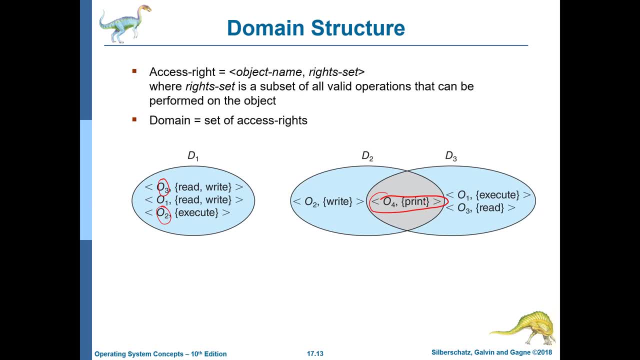 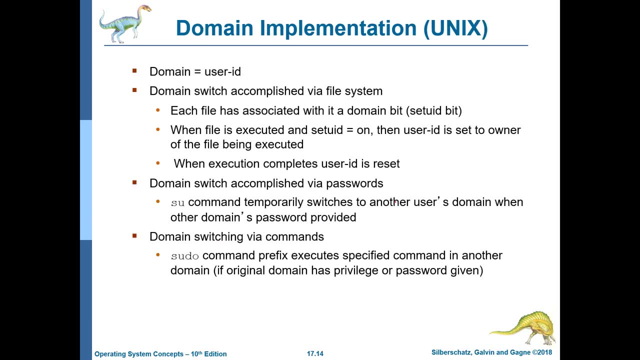 domain. these domains, D2 or D3, can issue this operation on object O4.. So how is the domain implemented in UNIX? So the domain is nothing but the user ID. So every user has a name, but a unique user ID as well and any kind of a domain switch. 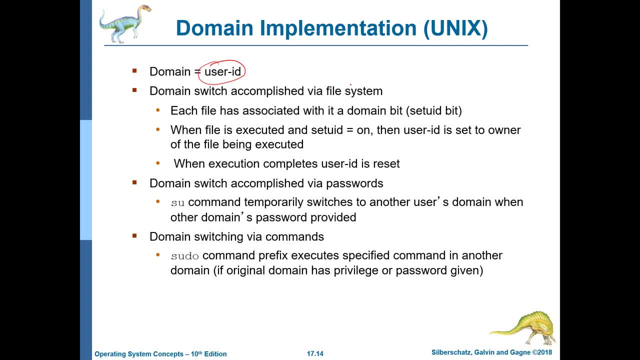 is accomplished by the file system. So every file has associated with it a bit called the set UID bit and when the file is executed, for example, the user ID is set to the actual owner of the file as per set UID, if set UID, if the set UID bit is on, which means that by default, if I am creating a file, 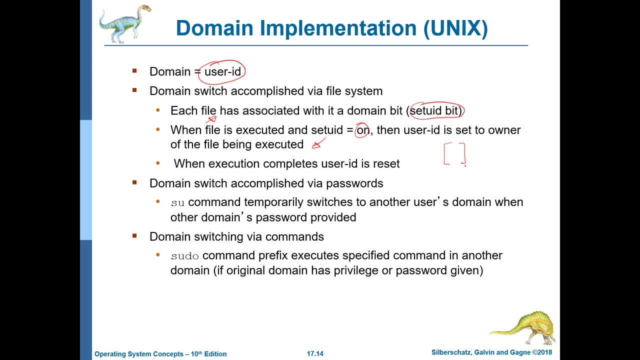 and I am executing it, then I am the owner. But it is also possible to execute a file as somebody else, particularly if the set UID bit of the file is on. So in this case I will be executing the file, but in the name of somebody else. that 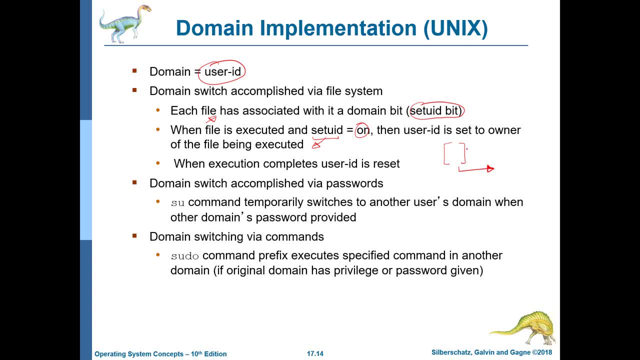 is if that somebody else has given me permission. So when I create a file, what I can do is I can give it permission by a mechanism called the sticky bit, and that basically means that when I am executing the file, when anybody else is executing the file, that person would execute with my permissions. 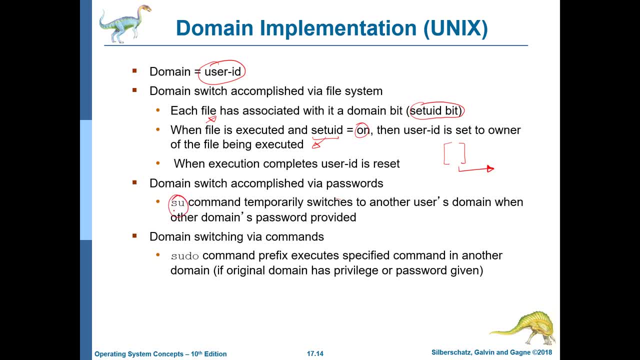 Furthermore, we can use the su command in Linux to shift from, let us say, one user to another user. So if I little say su username, this basically means that I want to login to the same system with the username of the other user. along with that, I can always just run the su command. 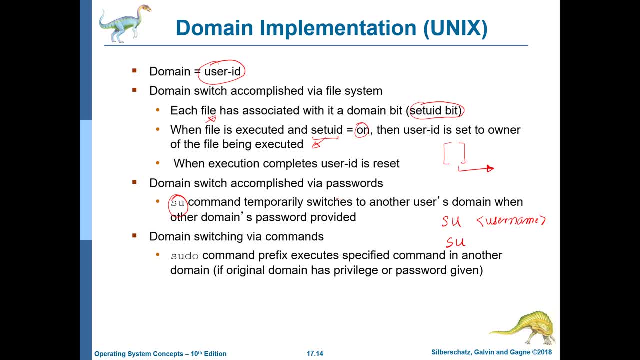 like that, which means that I will switch to. I will switch user- that is what su stands for- to the root and Linux called sudo. So sudo basically says that if I have sudo access, I can run a command and the system will perceive it that the root is actually running the command. 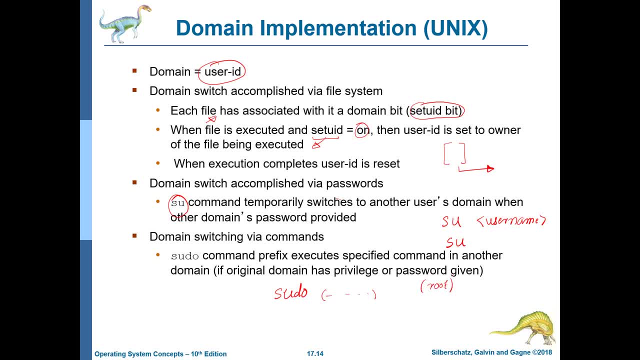 So the root is the administrative user, is the most powerful user, is the super user in the Unix Linux world. So in every Unix Linux system there is always a user called root which has power over large parts of the file system. 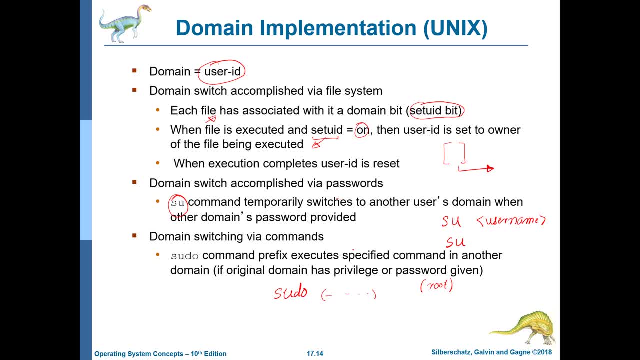 and can, for example, change the kernel or load a new module of the kernel. So the root is like the owner. So even normal users can be given some access, in the sense that they can be given access to some programs, for example, where they can run it with root. 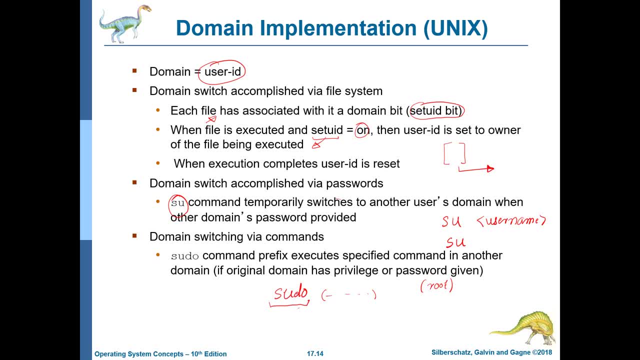 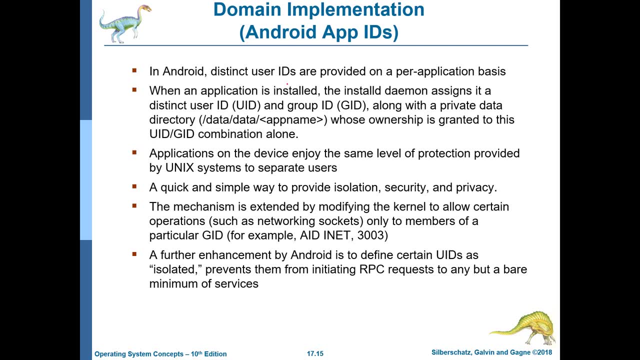 permissions, And the way to do this, other than set UID, is to actually use the sudo command. So Android's protection works slightly differently. So distinct user IDs are provided, in this case on a per application basis. So what happens is that when an application is 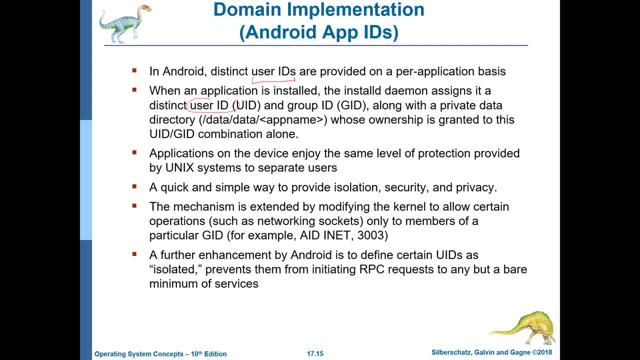 installed. the installer itself provides it a distinct user ID, a group ID, along with a private data directory where it can keep its data, which is slash data, slash app name, let us say, And the ownership is provided To this unique user ID, group ID combination, So applications that are running on the device. 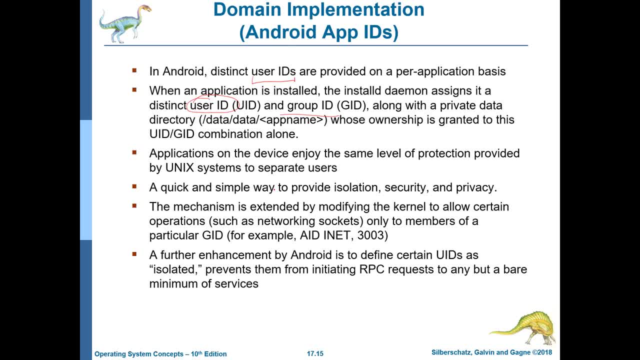 pretty much enjoy the same levels of protection that you would expect from a unique system And, furthermore, it is possible to restrict the services of the kernel or, let us say, any other service, let it be networking, or let it be the camera or anything- to a particular 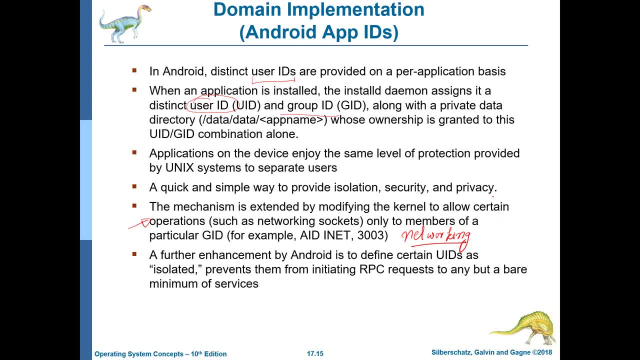 set of applications. So in this case, as I said, the idea is slightly different, The main reason being that, in any server machine, multiple users typically log into the server, But in this case, in the case of Android particularly, it is not the case that multiple users use. 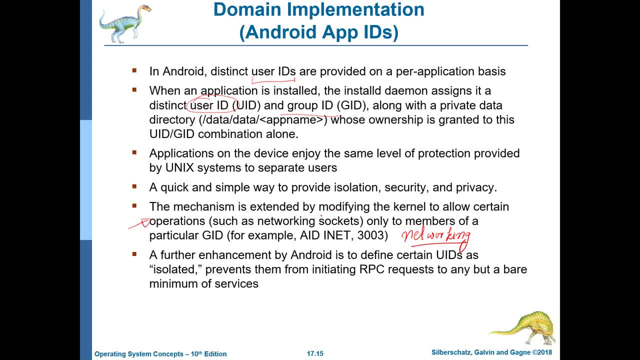 a phone, But we can think of each process as a user. Different processes, for example, can be accessing the camera or the networking subsystem at the same time. Consequently, they are our users. In this case, the process is the user And we can say that for networking, only these. 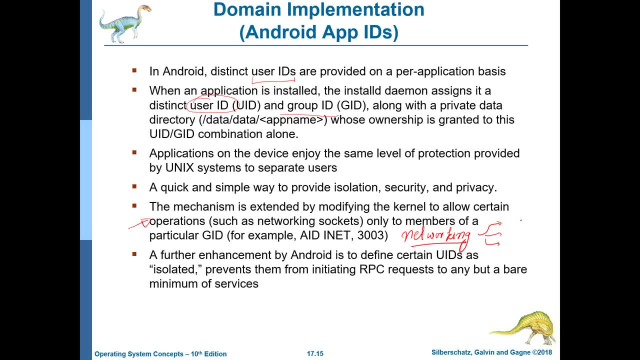 processes are allowed to access And the camera these processes are allowed to access. Furthermore, it is possible to define certain UIDs as isolated, which means that they will more or less not be able to do anything Other than a very minimal access to services. they 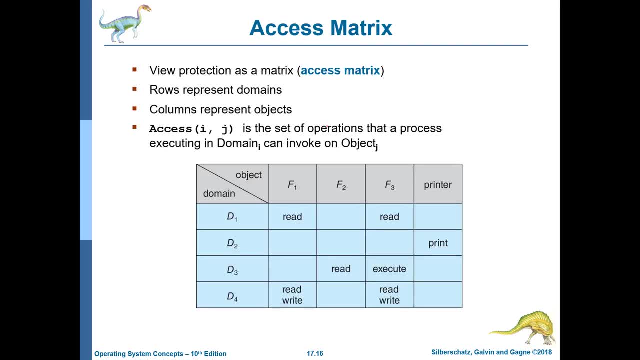 will more or less not be able to do anything at all. So now coming to the next part, which is the process. So in this case, the process is the user, And we can say that for networking, only these processes are allowed to access. 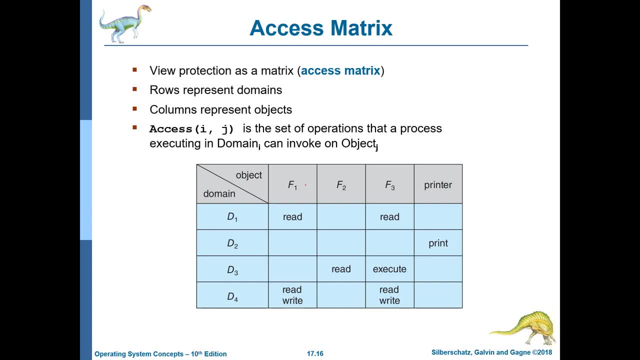 Now coming to the first mechanism. so we did talk about two mechanisms. First is the access matrix and the other is the capability model. So let the rows represent the domains, So domain D1, D2,, D3, D4, which are basically sets of users, basically, And the columns 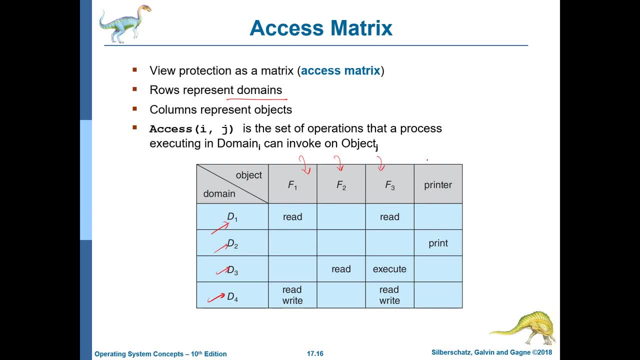 represent the objects. So the object could be a file, a printer, it does not matter. And if, let us say for a given row-column pair, what really exists is the operations that the domain can execute on the domain. So let us say for a given row-column pair, 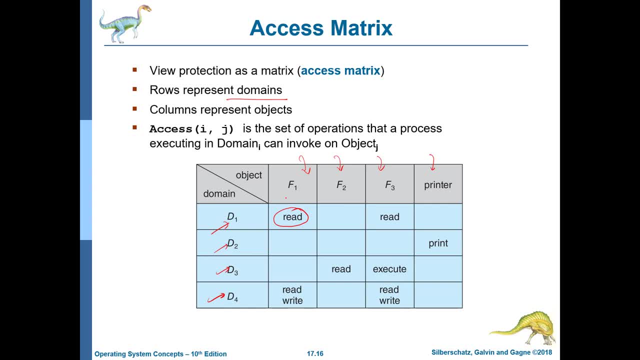 what really exists is the operations that the domain can execute on the domain, So this is known as an access matrix, which is in itself a fairly simple concept, And this is stored within the security subsystem of the operating system, And here this basically: 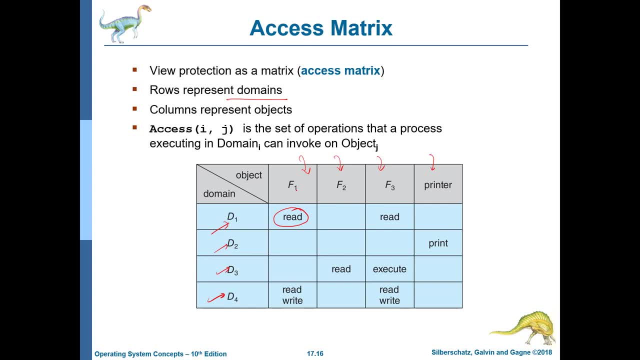 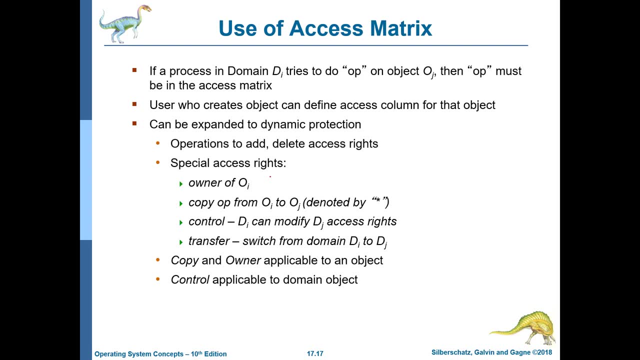 tells us which user can do what with which resource and also the operations that it can run on them. So what is the use of the access matrix? Well, anytime a user of a certain domain or a process in a certain domain can be protected by the access matrix, The 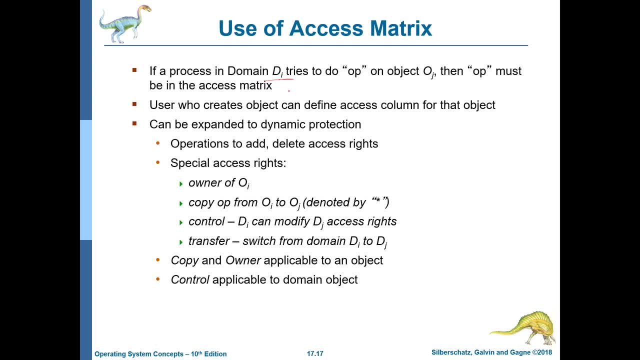 tries to access a certain object, then the access matrix can check if that operation is allowed or not. Furthermore, the access matrix can be modified. particularly, the owner of an object can definitely modify the access matrix and then permissions can be copied. and if, let us say, given domain, 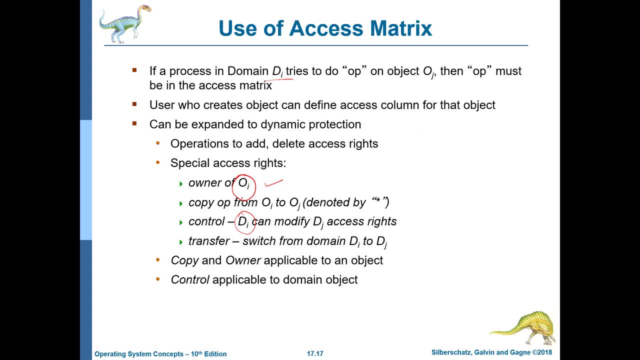 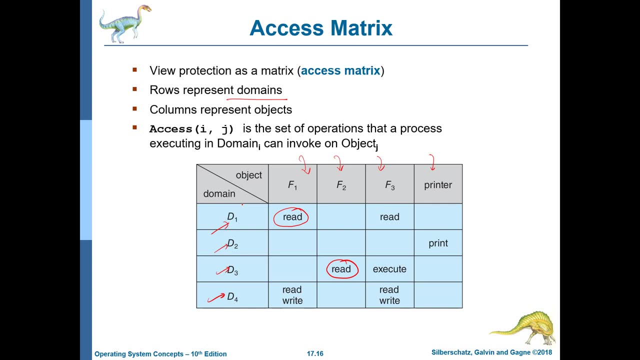 has the permission to change access rights, it can do so, And so there is a fair amount of flexibility over here in the sense how the access matrix can be configured. In a sense, you can have, let us say, one very powerful domain, like the root domain. that 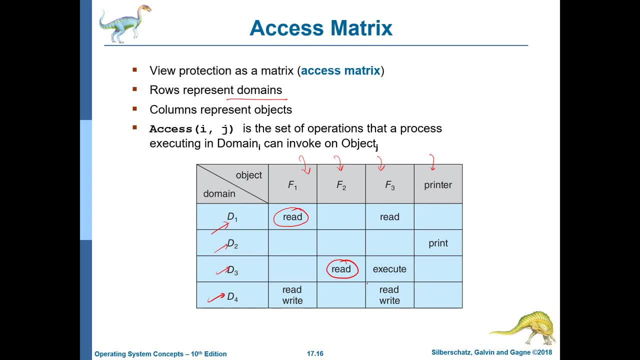 can go and change all elements of this matrix, Or you could have another process that can simply copy the permissions of one domain to the other. So there is a fair amount of flexibility. There is a fair amount of flexibility that can be given to a system to access and modify. 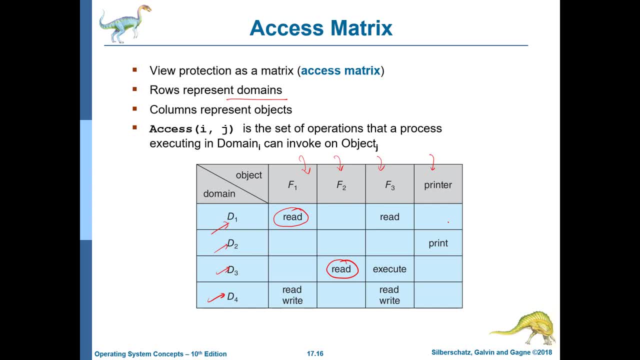 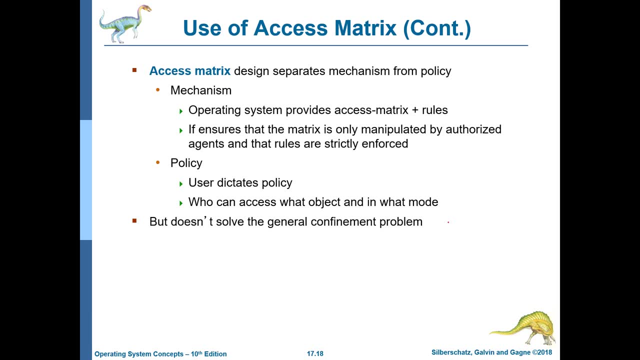 the access matrix. So the access matrix, as you can see, is a reasonably simple concept. So what is the mechanism? Well, the mechanism is the operating system maintains the access matrix and the rule: Only authorized agents are allowed to manipulate the access matrix and the creator of any object. 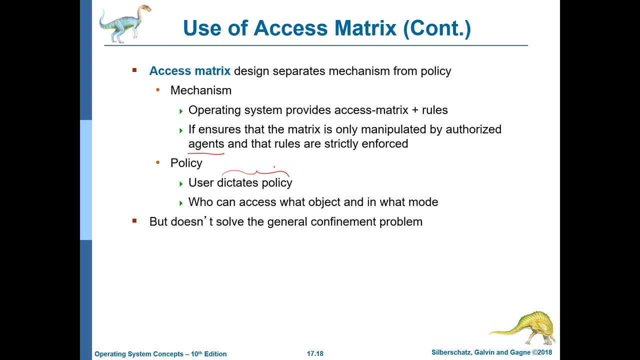 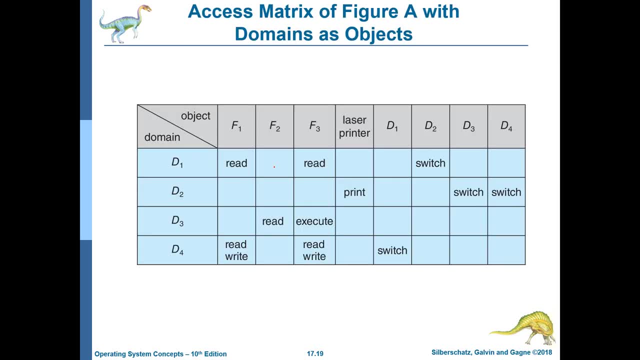 pretty much dictates the policy. So it dictates who are the other processes or other users that can access the given object. So what we can further do is that we can also have domains as objects, in the sense that if, let us say, I am in, I am a user in domain 2, I can switch to domain 3.. 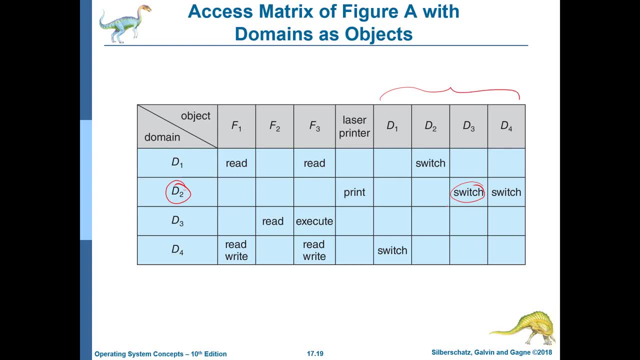 So I can also treat the domains as columns or objects- Fair, of course. What you will have is that it will just specify whether I can switch from one domain to the other or not. Furthermore, we can have an access matrix with copyrights. 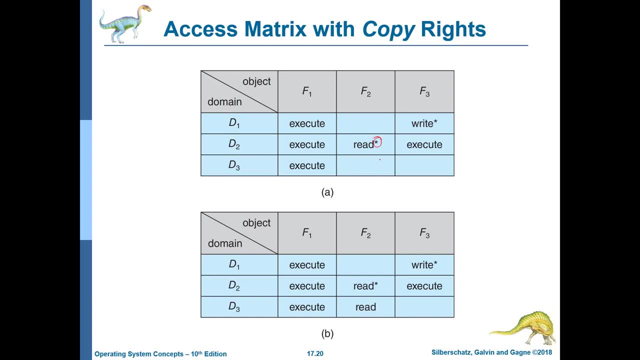 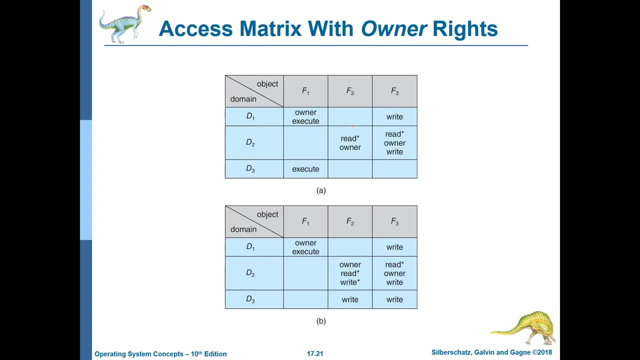 So, as you can see the star over here, give the rights to copy. This basically means that domain 2 can copy the permission that it has for F2 to other objects as well. Similarly, we can also have an access matrix with owner rights which can basically say: 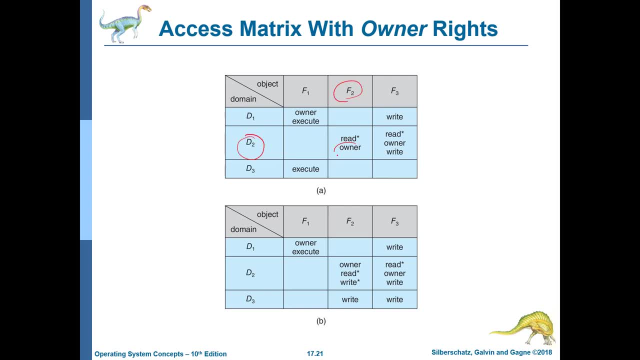 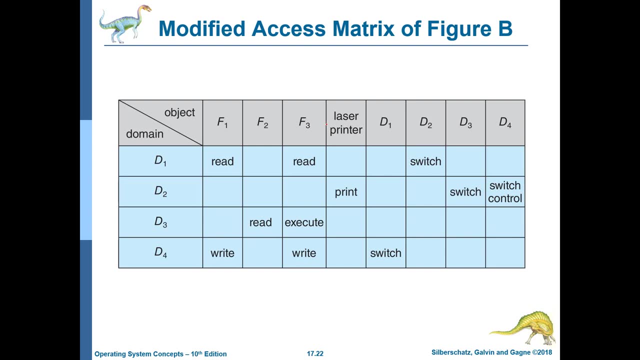 that domain D2,, for example, is the owner of F2. So we could add the owner information over here along with the permission copy information. So then, given the fact that we can have, we can sort of generalize this access matrix. 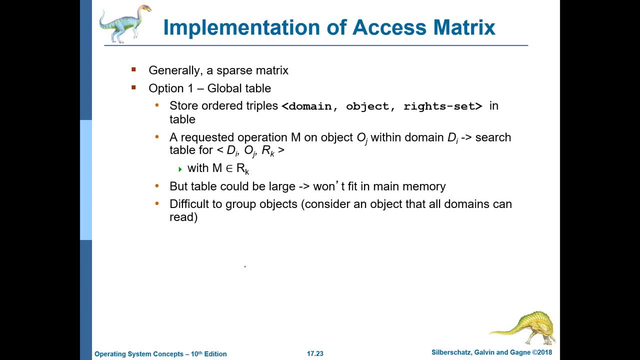 there is a lot that operating systems do to actually store, maintain and maintain the access matrix, So it is generally a sparse matrix, the reason being that we have lots of objects and lot of users, So it is not the case that we typically, for every user object, pair the access matrix. 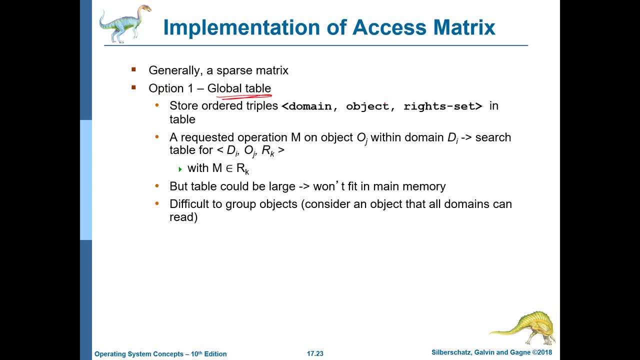 will have an entry. So one option is that we can have a global table where we store ordered triples of the domain, the object and the right side. So any requested operation: M on object: OJ with domain DI. all that you need to search. 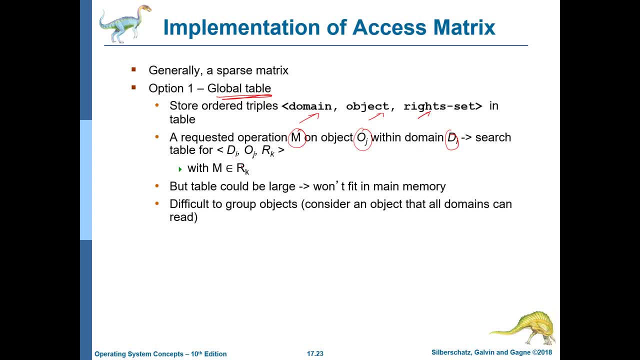 is that you need to search for DI, OJ and RK. So RK is the right set, basically where you want the operation to be within RK. So if you are able to find such a triple and, let us say, the operation you are requesting, 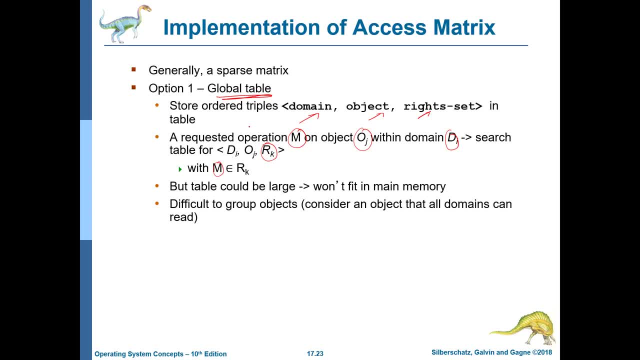 is within its right set, then there is no problem at all. the operation may be allowed. Unfortunately, this table can be very large and will not fit in main memory. And furthermore, to compress the table, we need to group objects. And furthermore, to compress the table, we need to group objects. 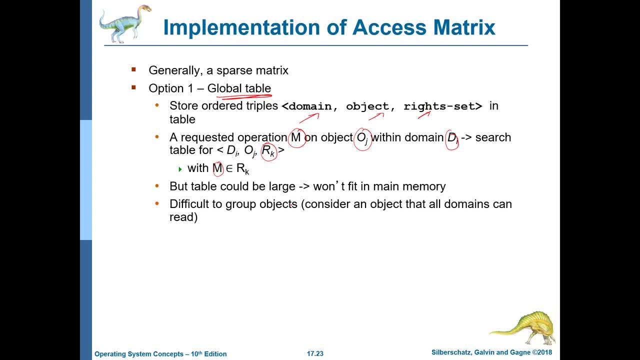 And for example, we might have one object that all domains can read. See, in that case we can omit a row of the access matrix. But in general that is hard. That is not. it is not that easy to recognize such patterns and also do something about. 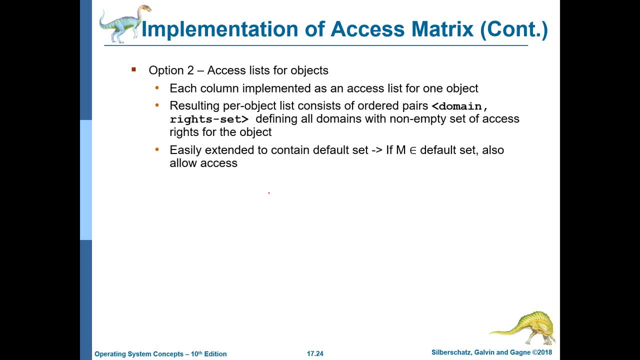 them. The other thing we can do is we can maintain access list for objects. See every column. if you think about it in access matrix, say: this is the access matrix and we have an object over here, so every column is like an access list for that object. so we can have for every. 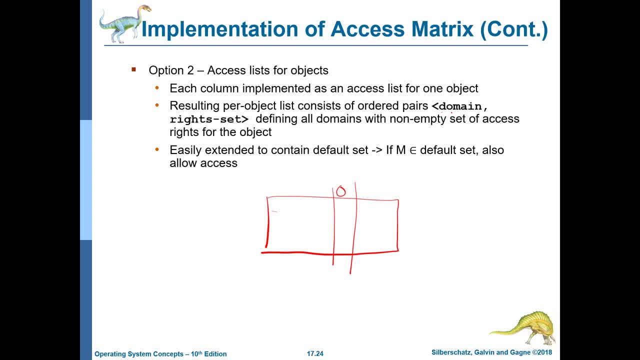 object. we can have a per object list which will be ordered, pairs of domain and write set which basically specifying all the domains and what they can do on them. so even if most of this is parts, it can just maintain a linked list of all the domains that have some rights on it. all right, and of course we can also have 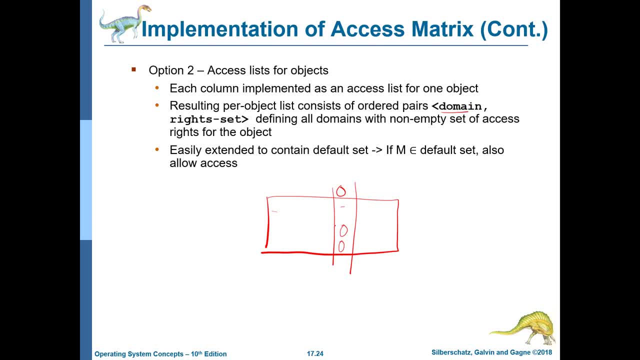 a default set, in the sense that if, let's say, I'm a member of some default domain, I will have access to this object. okay, so by? the key point over here is that, instead of storing the entire matrix, you can store it column wise and in each. 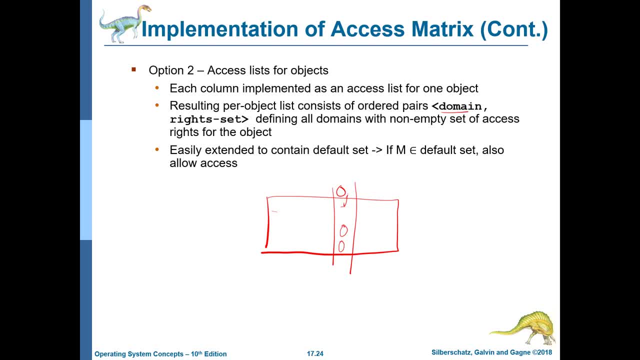 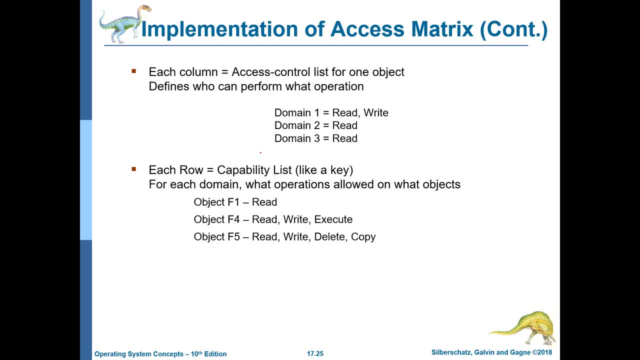 column, we can omit the entries that are empty and only store those entries which are non empty. so then in each column we, as I said, we can store. if you want to brush and we want to store everything, then we can store all the entries that are empty. so then in each column, the, as I said, we can store if you want to brush. 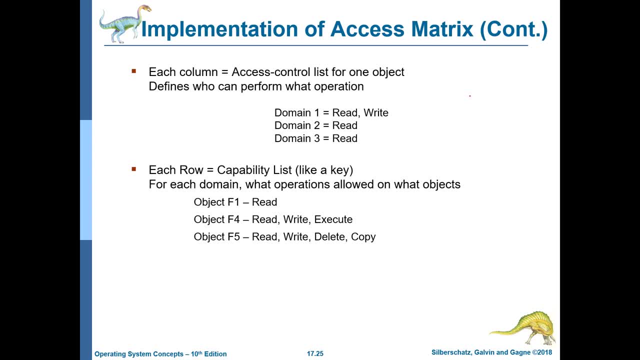 more compact storage we can store an access control list for each object, let us say for object oj. we will only set those access matrix entries which are not empty. So basically they may correspond to domain 1, 2 and 3 like: read, write, read and read. 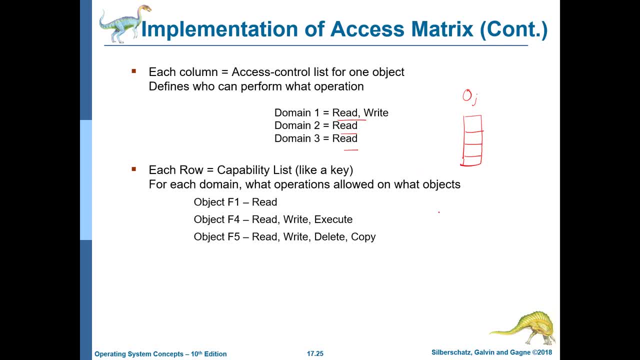 Every row is basically for a domain. so for a domain. if you look at every row of the access matrix, then it basically says that look for all the objects in the operating system, let us say from o1 to o n. what is it that you can do? may be some. you can read some you. 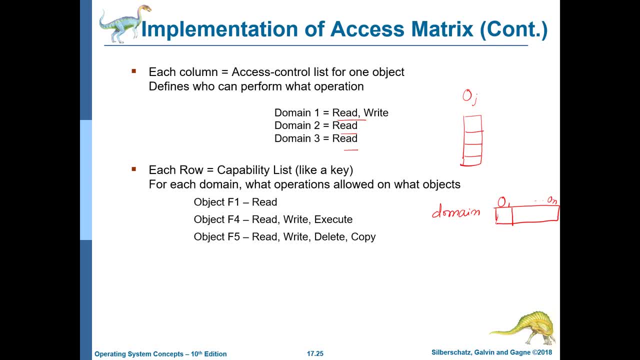 can read, write some. you can read, write and execute, say: every row of the access matrix is known as a capability list. this is a very important concept. it needs to be borne in mind that every row of the access matrix is called a capability list. 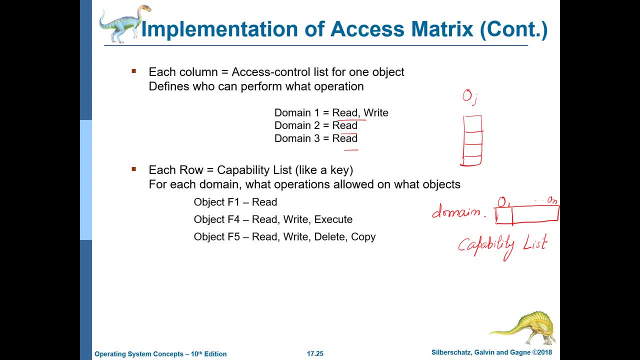 Why is it called a capability list? Because, in a sense, it is specifying. It is specifying the capability of a domain, what exactly it can do in terms of all the objects that it can access, what exactly can it do in terms of reading, writing and executing. 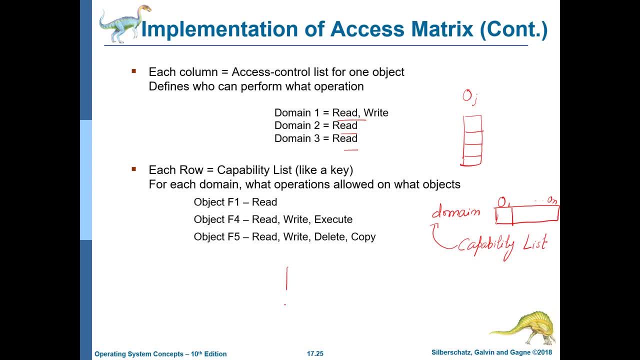 So the term capability list comes out of the access matrix. So the access matrix, if we split it column wise, then we can think of this as access vector for a given column. if we split it row wise, we can think of this as a capability. 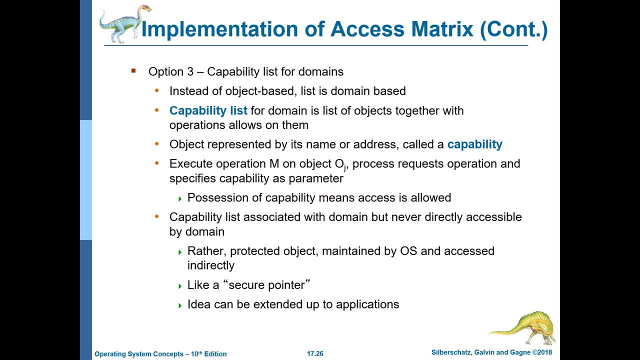 list for each object. So, expounding on this idea of a capability list for domains, if we create the list domain based, we will have a capability list for each domain and there again we can get rid of the empty or sparse entries and we can simply look at all the objects and the operations. 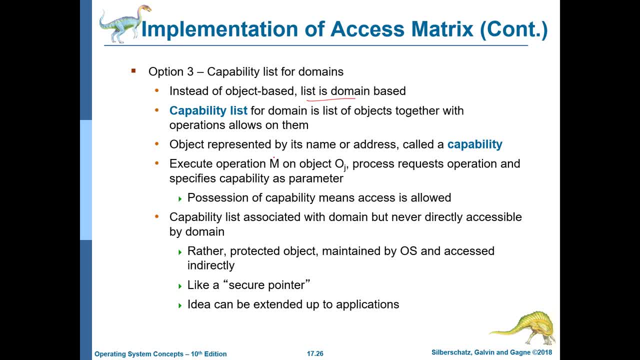 that are allowed on top of them. For example, if there is an execute operation m on object o i. so any time that a given process executes we just look at its capability list and if we see for object o i in its right set, is m an element of it. 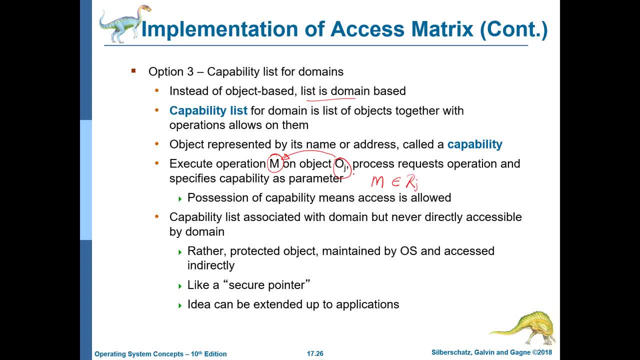 So we basically check if m is an element of the right set of object j. Any time I possess a capability, it means that that access is allowed. So the capability list is of course maintained by the OS, and so any object or any file pointer. 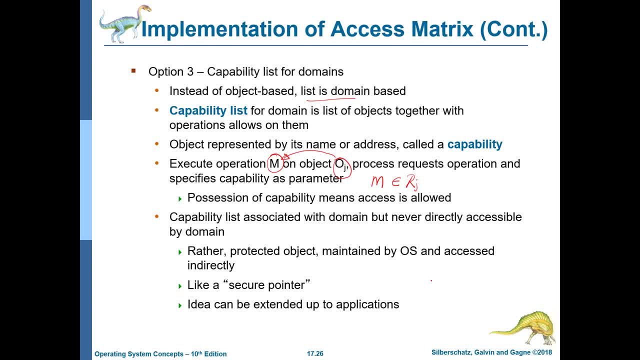 would contain another object. So again, another pointer within it, within the data structure, to the capability list. And so sorry, the capability list is per domain. so any time I make an access for a given process or a given user, my capability list will be checked and if I have the rights, the access. 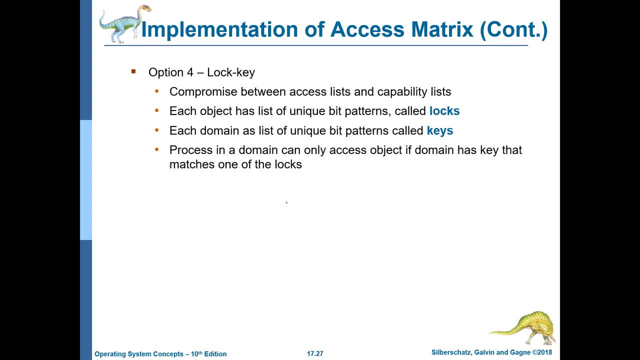 will be allowed, otherwise it will not. Another approach, which is like a compromise between access list and capability list, is like this: So recall that an access list is per object and a capability list is either per user or per process, any one of them. 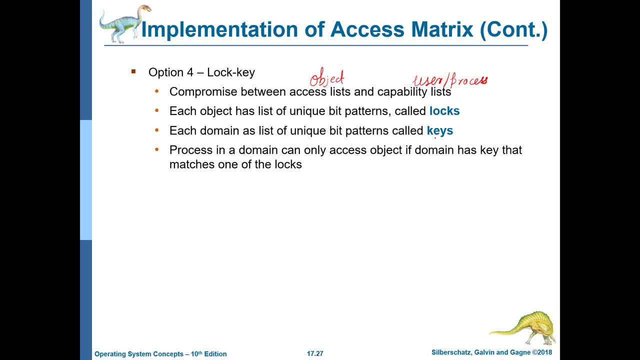 So we can have a unique bit pattern called a lock and another list of unique bit patterns called keys. Any process in a domain can only access an object if that specific domain has a key for that object. So what we do is that for every object, instead of maintaining an explicit list, we basically 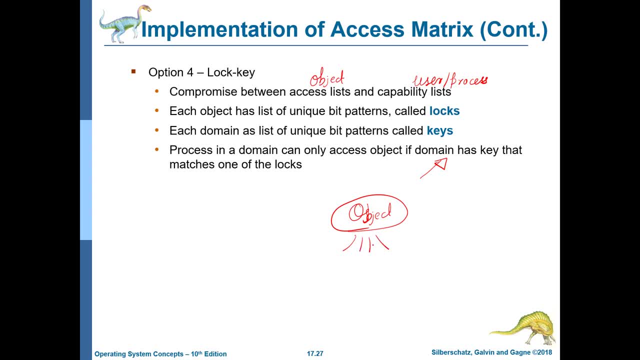 maintain a set of locks with an object. Any time a domain shows up and it wants to perform some kind of an operation on an object within the domain, we search for a key. So domain might have a set of keys. Essentially we try all the keys on the locks. 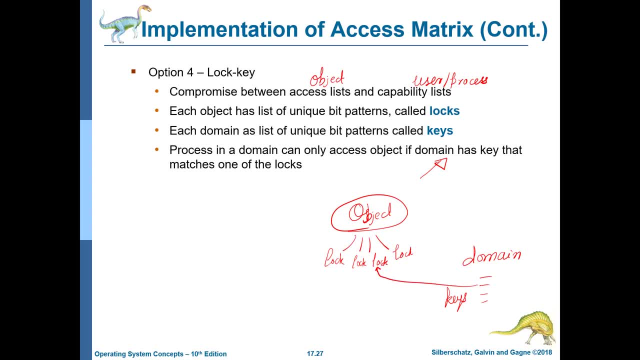 And let us say one key. If the key matches a lock, then it means that we have the access. So the domain can then perform the operation on the object. So of course the lock and key mechanism can take different amounts of sophistication. 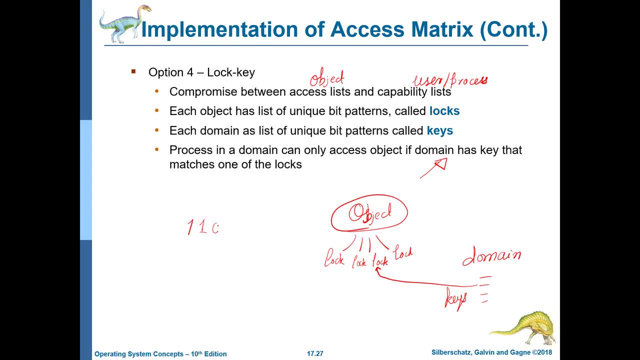 So one simple thing is that this could be, let us say, the lock could be a large bit vector with zeros and ones, And the key could simply be its complement. So in this case, all that we do is to check if the key matches the key. 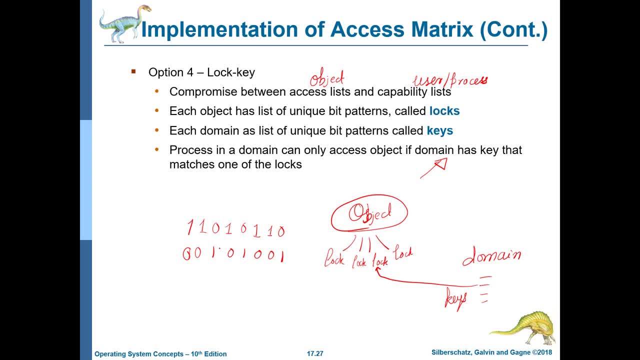 If the key is for a lock, we just take an OR of both of them, a bitwise OR, And if, let us say, the final value after a bitwise OR is all ones, then we are sure that this is the lock for the key or the key for the lock. 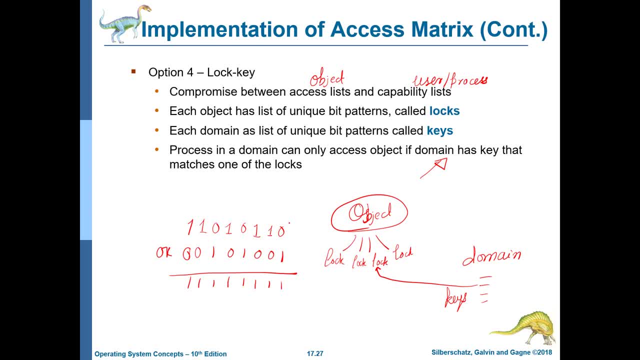 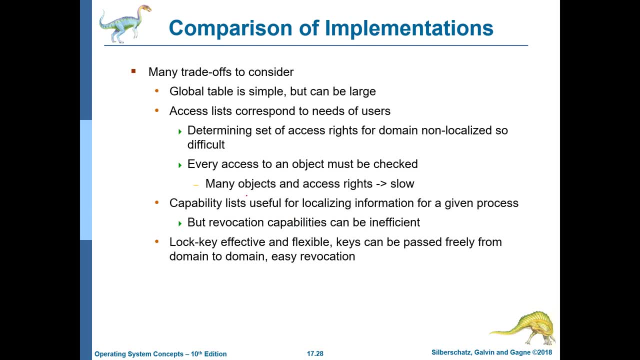 This is a slightly sophisticated idea when it combines the best of both the access list and the capability list. So, if we compare the implementations, having a global table is simple but it can be very large. An access list is great from the point of view of a user. 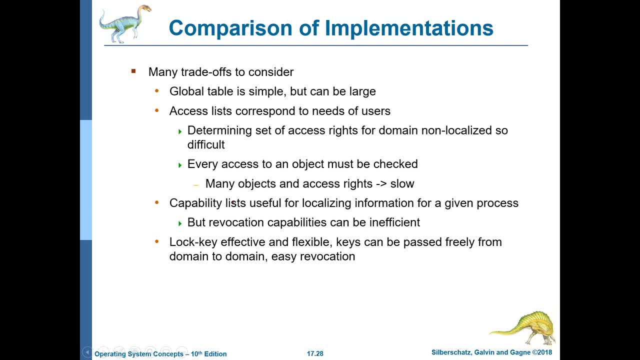 The reason why we say so is like this: Anytime that the user wants to access an object, all that it needs to do is that, for the object, it needs to look up the access rights and then basically see if it has the rights or. 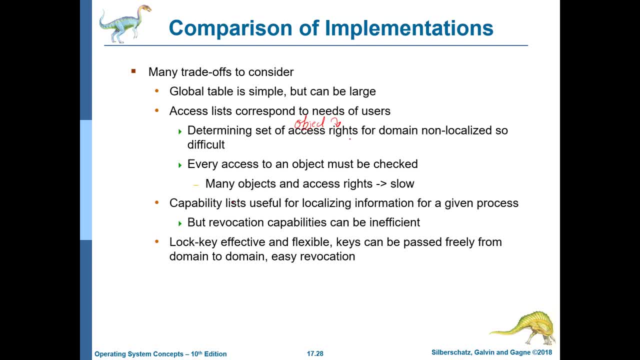 not. So of course we can have the issue of non-localized domains, Which basically is not a problem, Which basically means that if we have a network system where I have accesses to another machine but the other machine may not recognize the domain I am from, that will cause somewhat. 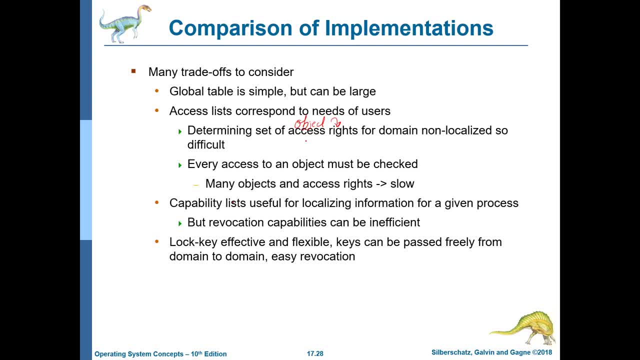 of an issue, but we can always fall back to a default. The only problem is that every access to an object has to be checked. If you have an object with a very intricate set of access rights, it can be slow. Capability lists, on the other hand, are useful. 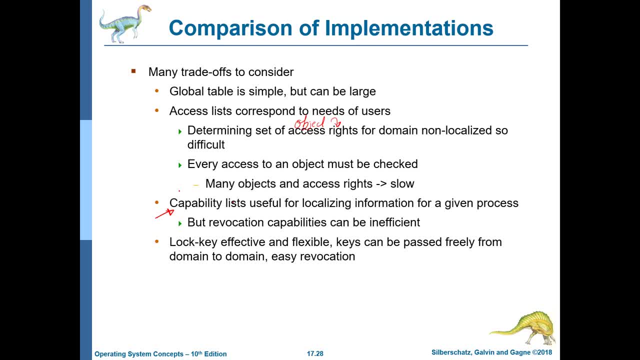 They are useful for localizing all the information of the given process. So anytime that we actually run a process, what we can do is we can load its capability list into memory and then quickly check if it has access to a given object or not. 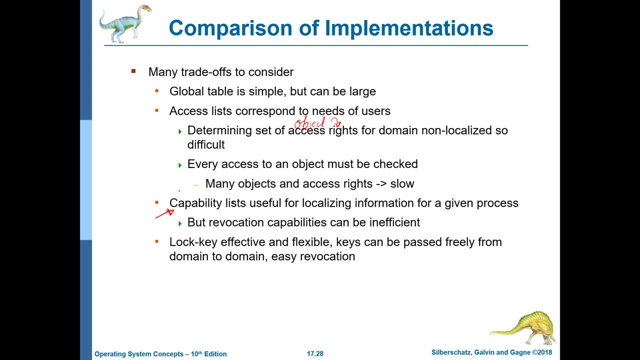 Of course, revocation capabilities are more difficult in the sense that let us say that I want to maybe ensure that no process has execute access to the object. In the case of an access list, it can be done very easily in the sense that I go to the 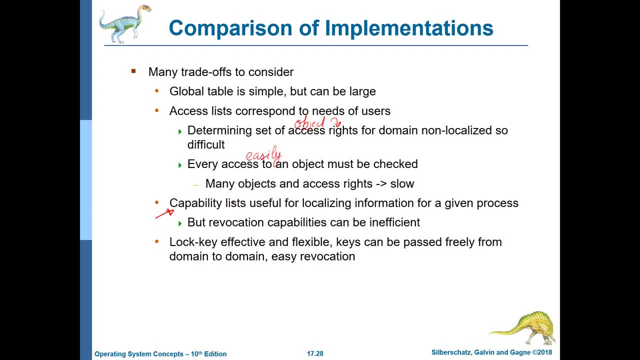 object and simply take out all the execute permissions For the capability list based approach. what I need to do is I need to look at the capability lists of all the processes, all the domains registered in the system, and remove this permission from them, which can be quite inefficient. 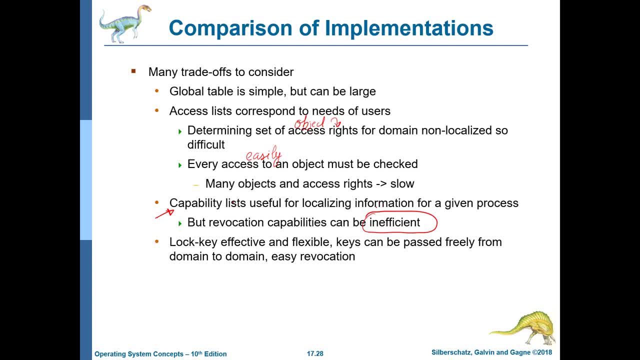 The lock-in key is effective and flexible in the sense keys can be shared. they can be passed freely from domain to domain. it is easy to revoke a permission, in the sense we can just change the lock and all the keys will become invalid. so that also is doable. 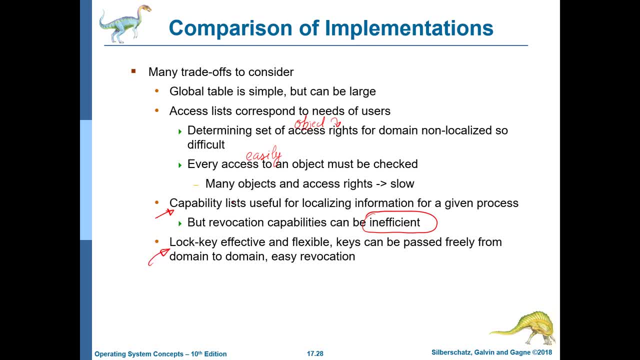 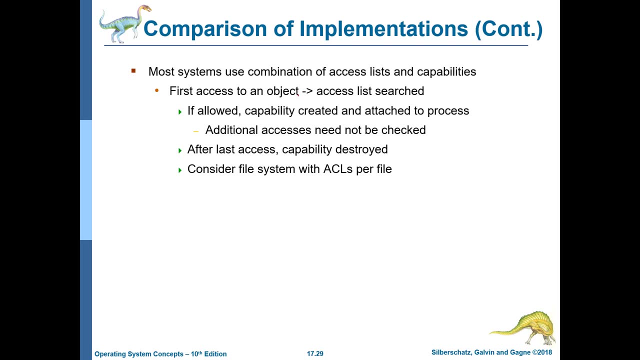 So the lock key method is fairly effective, but of course here the issue can be that if a key is stolen, then pretty much the malicious process has access to the object. So many systems, So I would say most systems, use a combination of both the approaches: an access list and 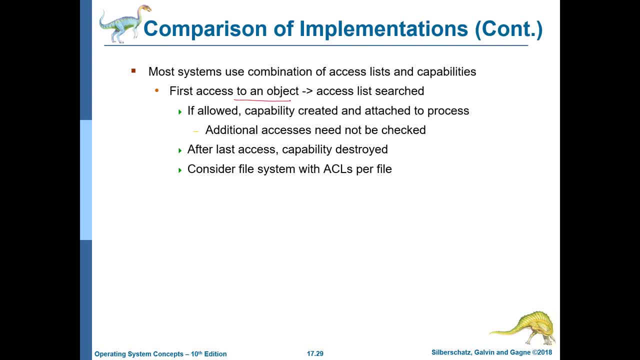 a capability list. First, you access an object, search its access list. if allowed, then a capability is created which is a data structure, a dynamic data structure. It is created and attached to the process such that for subsequent accesses or additional accesses, nothing needs to be checked. 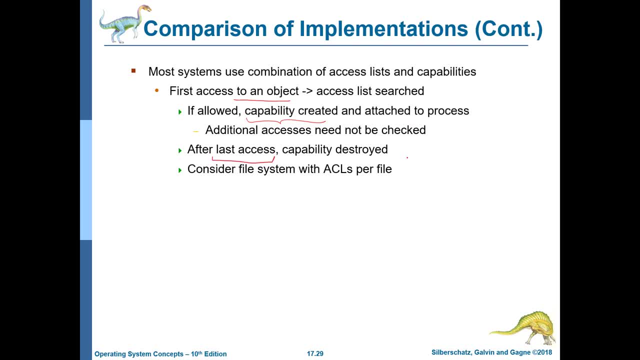 After finishing the last access or after, let us say, one or two accesses, nothing needs to be checked. So let us say, while terminating the process, the capability is destroyed, and this is something that is done in files to a large extent, that the first time we access a file, we actually 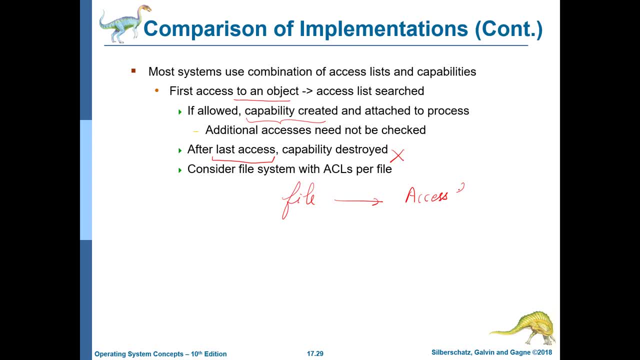 check its access list. So it is less intricate on Linux and more intricate on Windows. See if, let us say, if the given user or the given domain has access to it, well, that is great. So then we create a capability out of this. this capability is attached to the process. 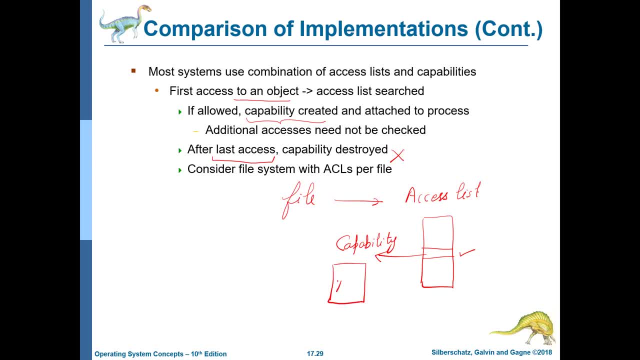 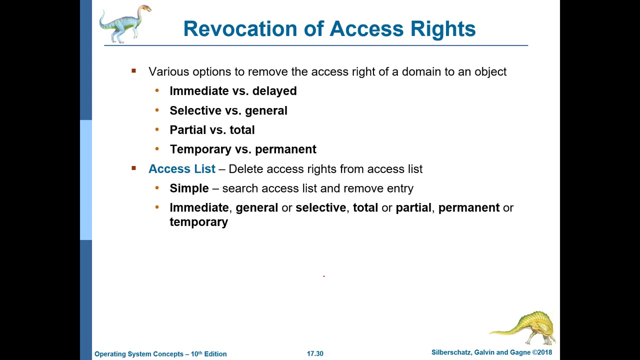 and given the fact that this capability is attached to the process, what can be done is that for any subsequent access to the file, you do not have to check the access list once again. So this capability is good enough To revoke access rights. well, there are various options. we can either revoke it immediately. 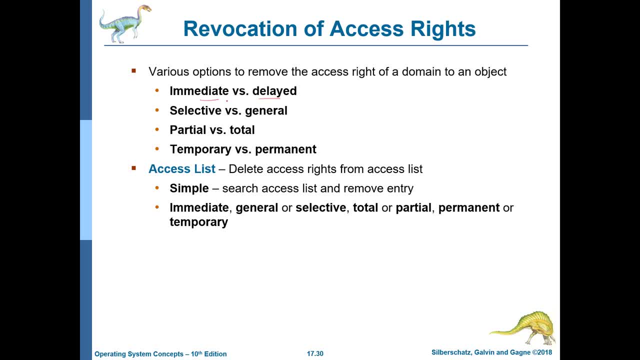 or delay. We can be selective while revoking it or just have a sledgehammer based approach: revoke everything- partial, total, temporary, permanent, With an access list, as we have argued. it is kind of simple, because all that we need. 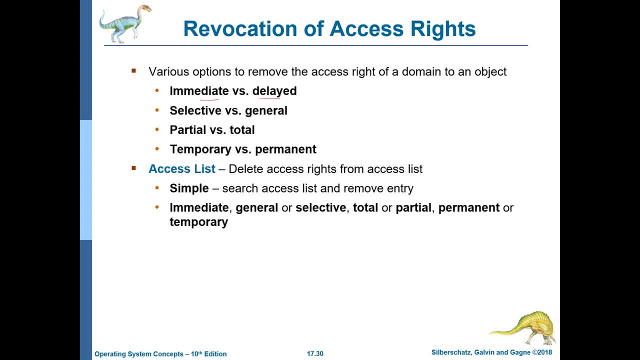 to do is we need to search the access list, find the entry and remove it, And of course, here it can be done immediately. We can either remove it for all the domains or maybe keep it for a few, and furthermore, maybe we can remove it on a temporary basis. 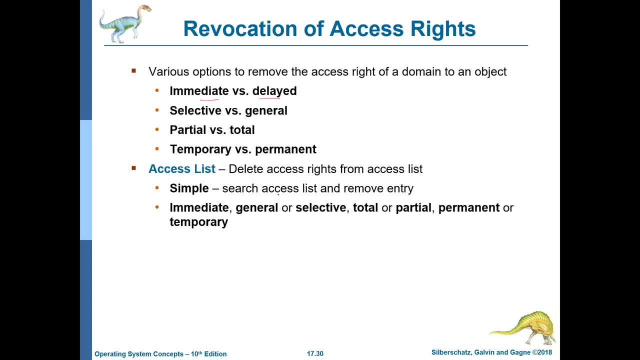 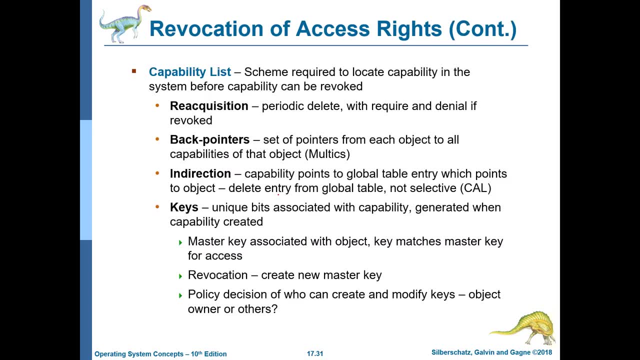 So we can say that, look, I am removing it for one week, but after one week it will get reinstated In the capability list scheme. revoking a permission is quite hard because we will need to check everything, check the capability list of all the processes or all the domains. 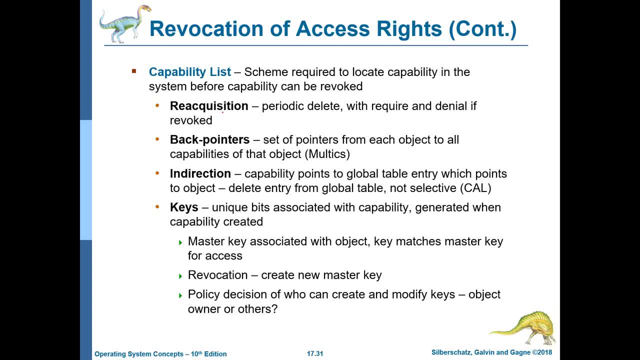 Domain is a more generic term here. So of course we can periodically delete. Then we can have back pointers. Okay, Back pointers in the sense that we can have a pointer, let us say, from the object to all the capabilities of the object. 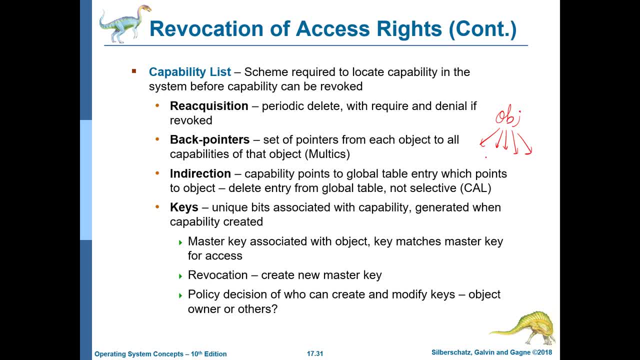 So these are called back pointers, like in the multi system. Of course this can be a fairly large set of pointers, but then the key point is that from a given object we can reach all of its capability lists and then delete the permissions. 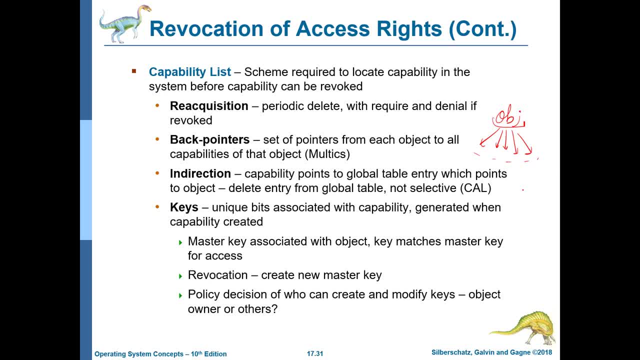 Or we can have an indirect capability list. A CL points to a global table And in the global table if we delete something then it will automatically get deleted in all the capability lists And of course the lock-in key method, or any extension of that, does work over here. 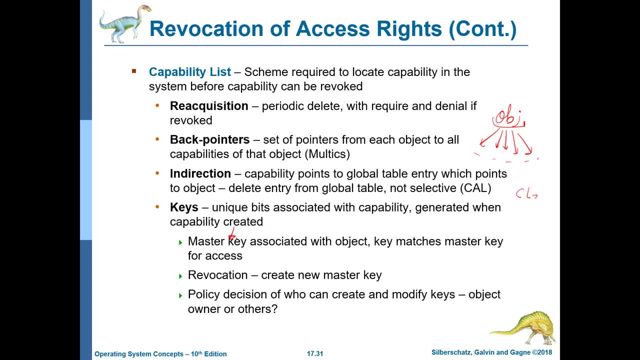 In the sense we can have a master key associated with an object And any time that I would like to access the object, I need to ensure that the master key matches. Any time I wish to revoke a permission? Okay, Any time I wish to revoke a permission, I can just change the master key, which is nothing. 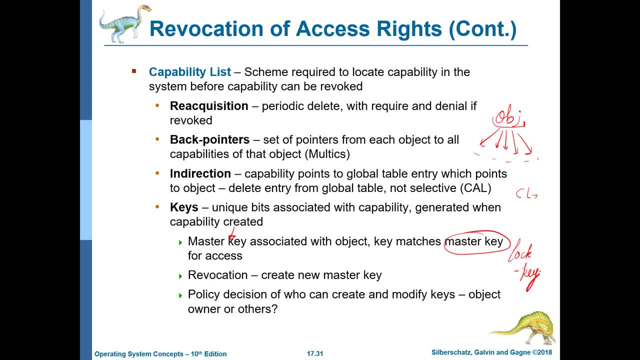 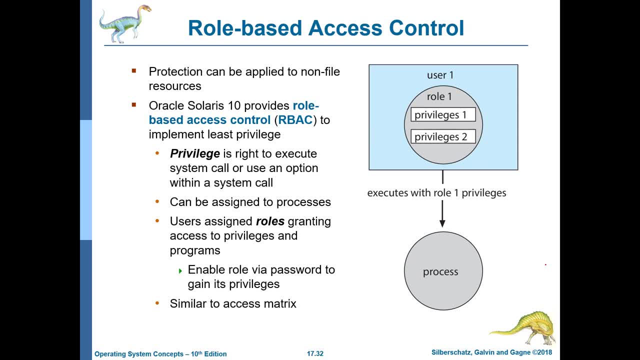 but a simple modification of the basic lock-in key based approach. Now coming to role-based access control, which slightly differs from domain-based access control, we can assign users roles and note that a single user can take on multiple roles. So, unlike other systems where a given user kind of has a fixed position in the hierarchy, 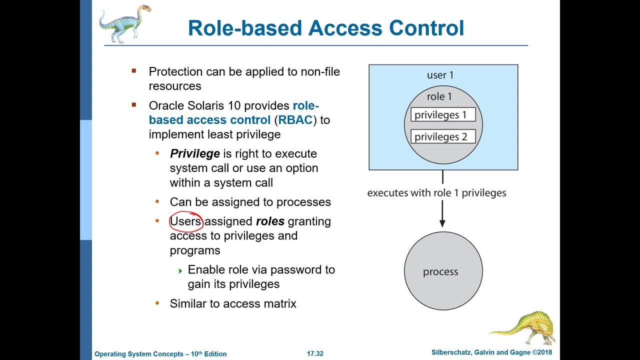 of users. in this case, the roles can also change. So let's say, user can be a manager or can be a senior manager or can be a vice president, and that will enable the user to access a broad set of resources. 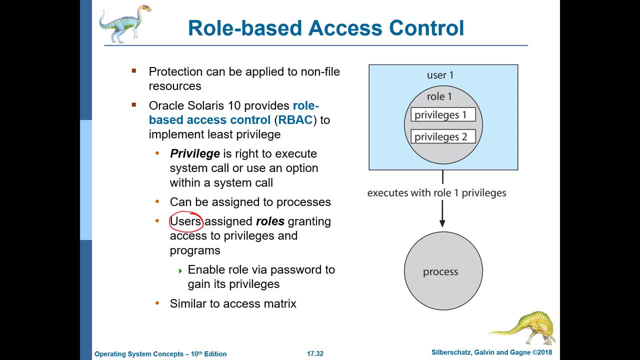 So this is something that Solaris uses. So, for example, the role can be changed via a password such that the same user user remains the same, but the role changes, So the user can now access more objects. Okay, 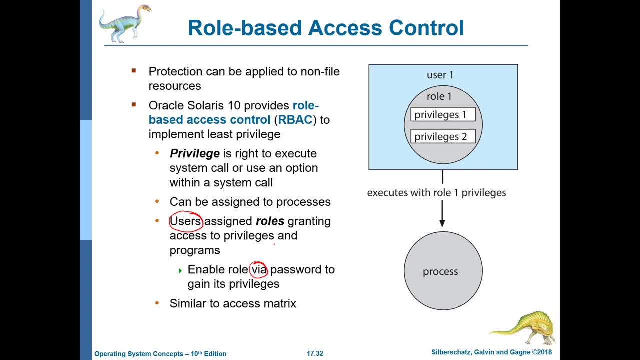 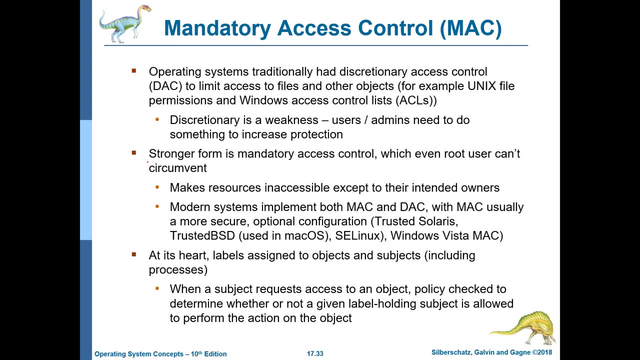 Similar to an access matrix broadly conceptually, but the key idea, of course, is that what is the capability of a domain that dynamically increases or decreases depending on the role? Then we have some other systems called mandatory access control. So operating systems traditionally have followed what is called discretionary access control. 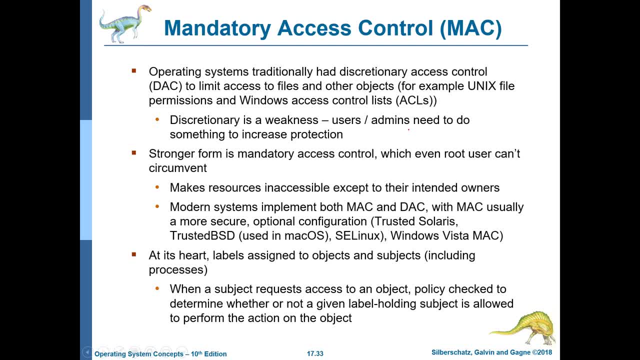 which means that every object has a set of permissions, Every user may have a set of capabilities which are dynamically given to it, and they can increase and decrease and so on. but we could have secure versions of an OS like a secure OS. 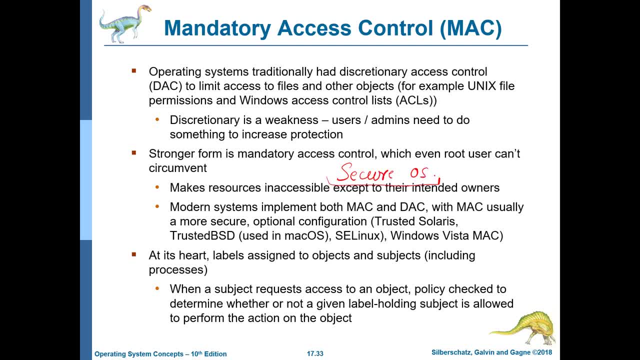 What the secure OS will do is that it could be hardwired with the access matrix. basically could be hardwired in the sense that every object will have a set of labels and every subject will also have a set of labels. Okay, So it's like a lock-in key, but it's like a hardwired lock-in key. 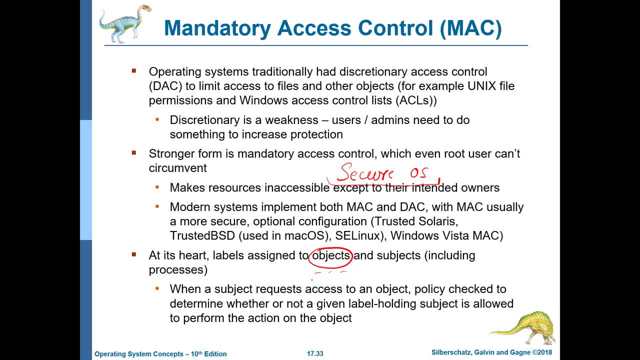 So, whenever the subject requests access to an object, you find whether the labels that the subject holds, like the keys that the subject holds, are compatible with, let's say, the locks that the object holds, and if there is a compatibility, then the subject is allowed. 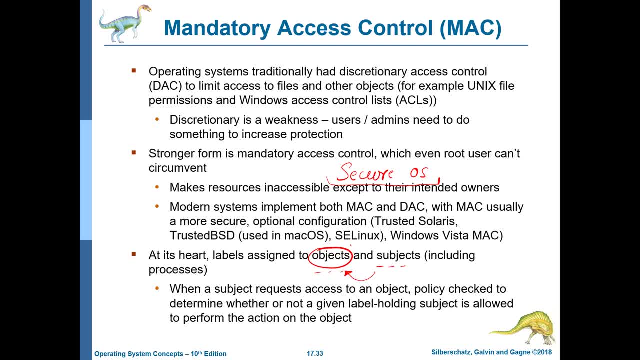 to access the object. otherwise it is not, and most of the time these capabilities are not changed during the execution of an operating system, so it's much more hardwired in that sense. So of course a general purpose system cannot be that inflexible. but this idea of a mandatory 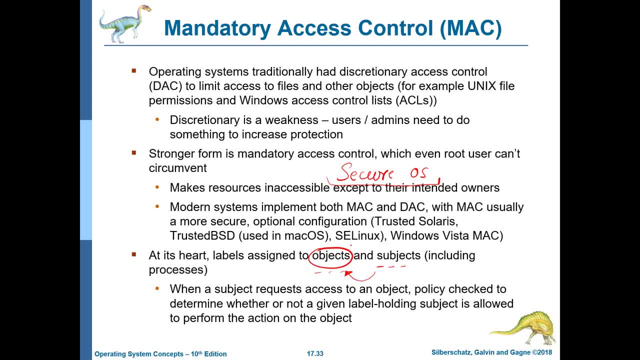 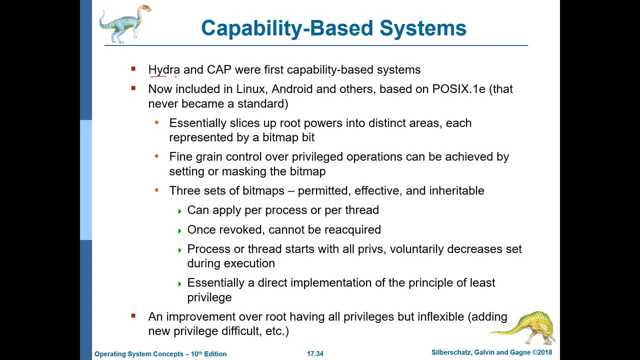 access control is a reasonable choice for a secure operating system where we don't really expect capabilities, domains and roles to change, Coming to a capability-based system. So Hydra and Cap, which were like early operating systems, were capability based systems. 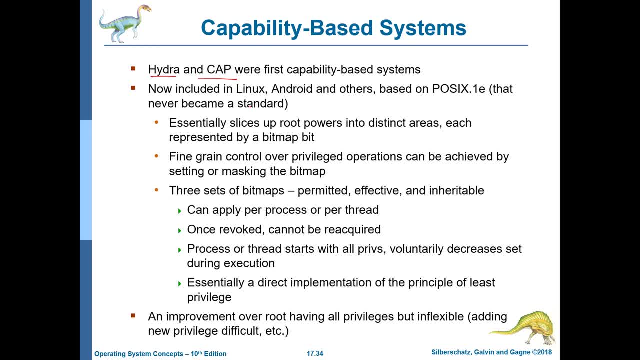 Linux, Android, have some notions of capability, even though they are primarily access-list based. So basically, what we do is that we do give fine-grained control over certain privileged operations by creating bitmaps. So every processor has three kinds of bitmaps. 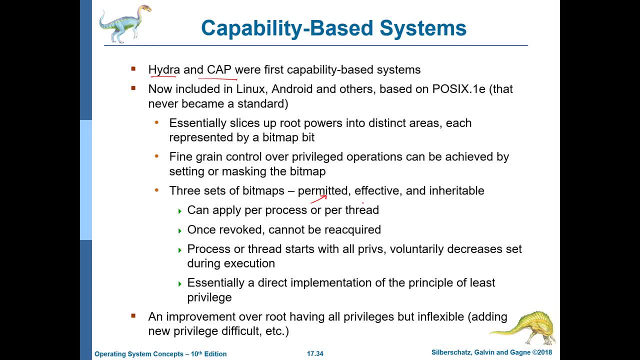 maps permitted, which means what all it is allowed to do, effective and inheritable. So this we can apply per process or per thread, and they of course, can be revoked and can be reacquired. So what happens is that whenever a process or thread starts, it starts with all privileges. 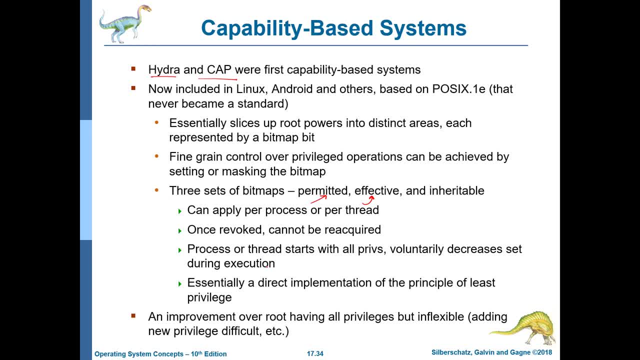 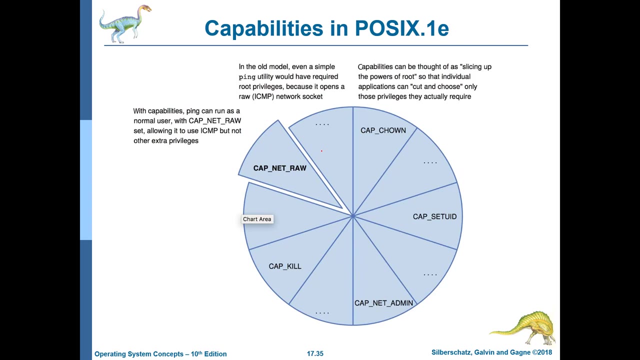 but during its execution, if it does not need something, it reduces it. So, essentially, the implementation of the principle of the least privilege. this is something what it can do, and then dynamically it reduces itself such that, just in case it is taken over by an attacker, it will not be able to do much. 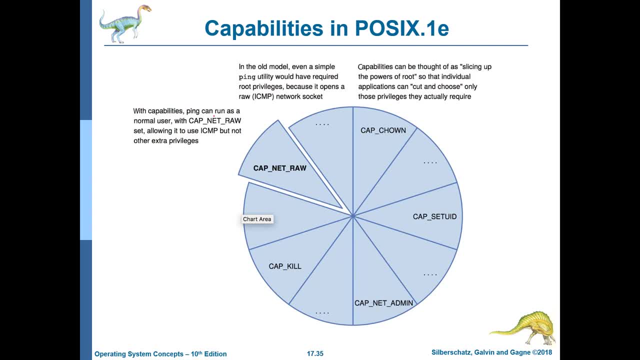 In any POSIX based system we have some standard system calls to increase or decrease capabilities. So, for example, you can say that, look, certain network protocols can be used by certain processes and certain processes cannot use a certain set of network protocols. For example, let us say the ping utility, which is just needed to ping if a machine is alive. 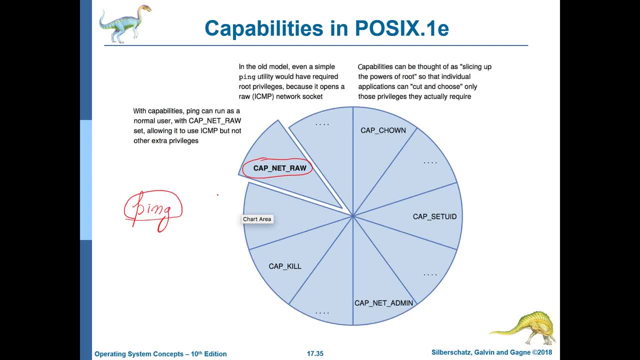 or not. maybe that is all that I will give to a process. I will not really allow it to communicate any more data on internet, but all that I am willing to do is to give it to a process, So this can be allowed. Furthermore, we can say that I can give it the capability to, let us say, change the ownership. 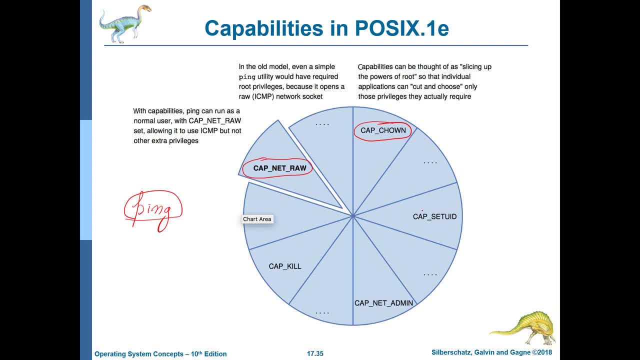 of a file as long as the file is not owned by root, or I can give it the capability to set the UID of a file, in the sense it can create a file, making itself the effective user. So let us say: this is user A and another user B actually executes this file. the file will 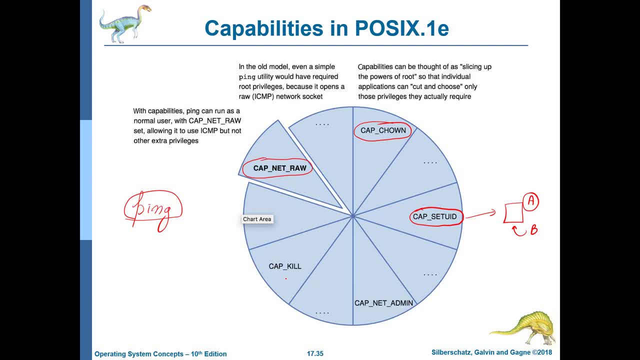 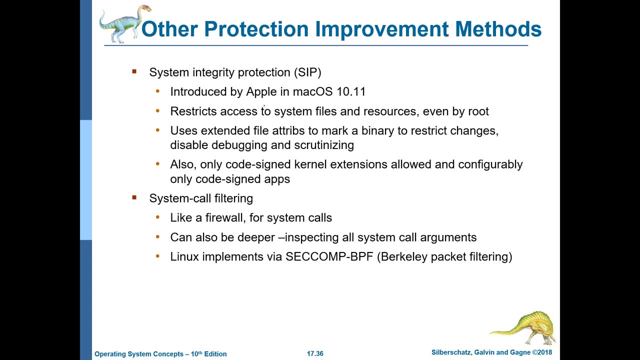 run with the permissions of user A and similarly in other capabilities can be given whether it can kill a process, whether it can perform network administration and so on. There are other improvement methods, other improved protection methods. So for example, in Mac voice there is a very elaborate mechanism to restrict accesses to. 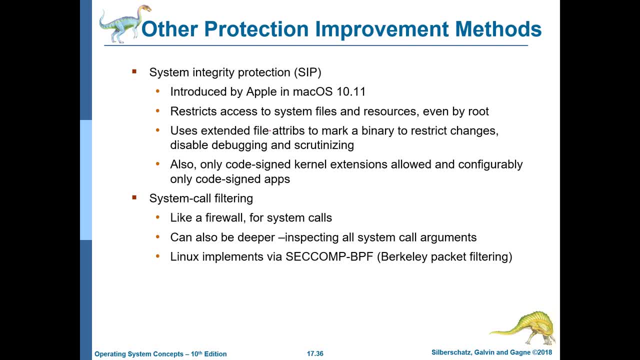 system files and resources. The key idea is that we extend the file attributes Okay, And we can control things like whether I am allowed to debug the code or not, because debugging allows you to scrutinize the execution and find out parts of the code. look at the register. 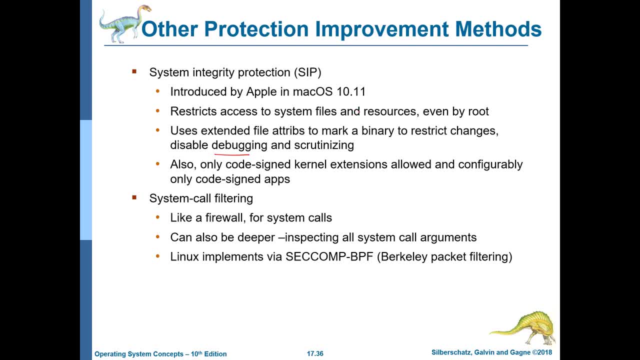 state: variable state: look at assembly code snippets. So this can be explicitly allowed or disallowed. Furthermore, let us say that if any kernel extension, like a kernel module, is to be installed, normally operating systems say that it needs to be signed. 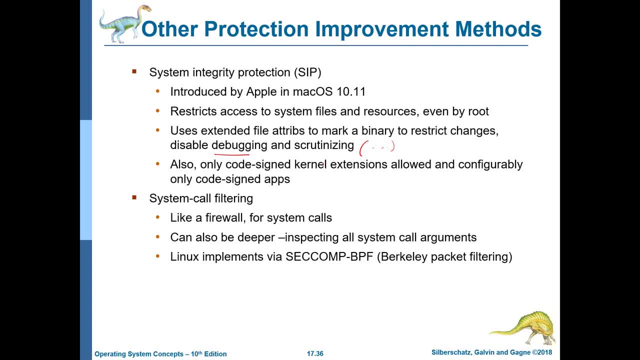 Signed basically means that we will only trust extensions from, let us say, the vendors. So in this case- maybe for Mac voice- we will only trust extensions from Apple and nobody else. So in this case, what Apple needs to do is it needs to sign the extension with its private 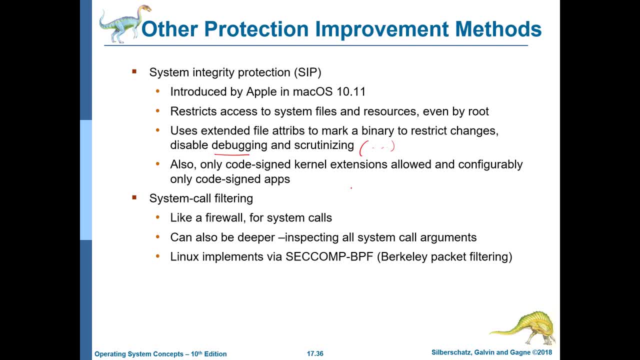 key, such that anybody who is installing the extension can decrypt it with the public key and verify that indeed, the extension is from Apple, Similar to firewalls. Yes, Yes, In the same way, you can also enjoy and check out your machines, Okay. 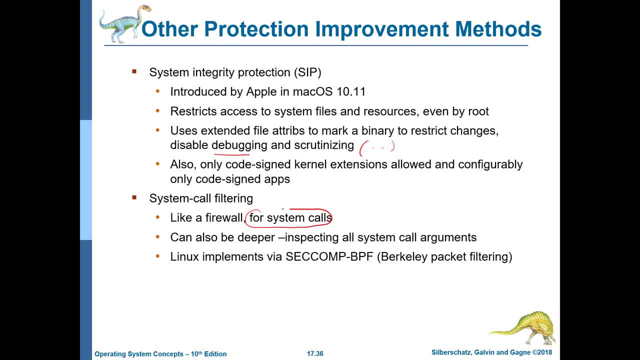 Okay, So we have seen the other DaVinci process that filters the network connection. We can also filter system calls. so this is there in many modified versions of Linux, where you basically say that certain processes can perform certain system calls and certain processes. 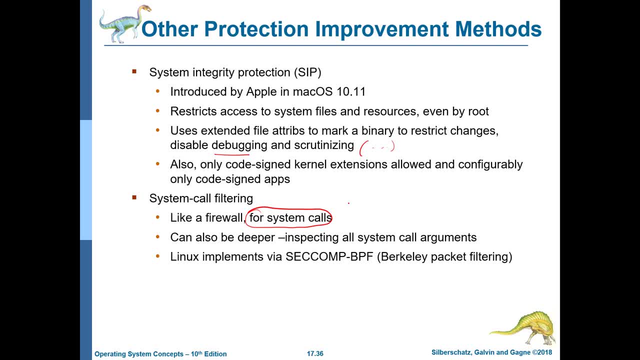 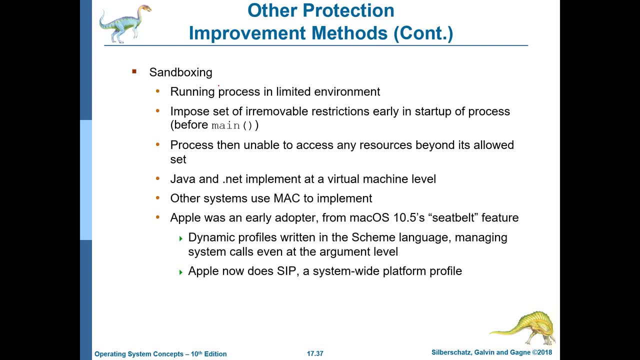 are prohibited from performing a few more, few other system calls. So this idea has been extended in what is called sandboxing, where we run a process in a limited environment or in a controlled environment, and the controlled environment is basically called a sandbox. 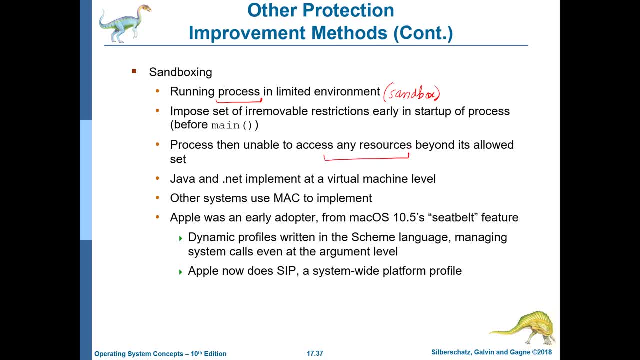 So then, what the sandbox does is it limits the resources that a process can access. So this is very common in Android. So, for example, you say that the process can maybe access the camera, it can access the speaker, but that is all. it cannot access any other device. it cannot access the printer. 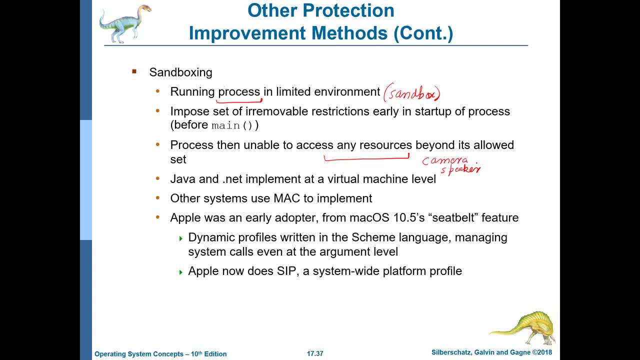 for example. So this is kind of leading us towards a virtual machine that basically looks at the program and executes it, not instruction by instruction, but allows the program to execute, but just traps the system calls and re-implements them. But the key idea of a sandbox is that it essentially traps all the system calls and accesses to. 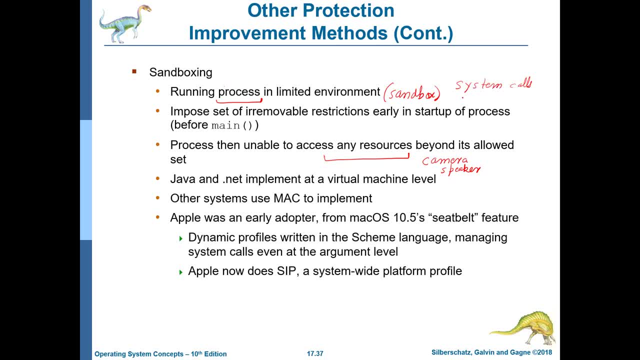 devices and then enforces a policy, So primarily system calls and hardware device access, And then the sandbox enforces. It enforces a policy of whether something is to be allowed or not. So then, macOS X went one step further and basically created what is called the seatbelt. 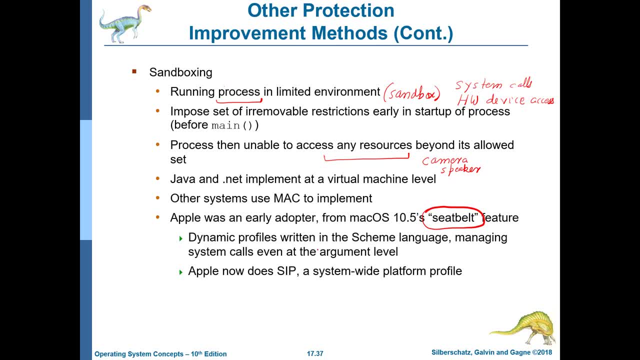 feature. This allows you to actually look at the arguments of system calls, allow certain arguments and disallow certain arguments. So there is a language called scheme. it is a functional language that allows you to create these small code snippets via which you can look at the argument of a system call. 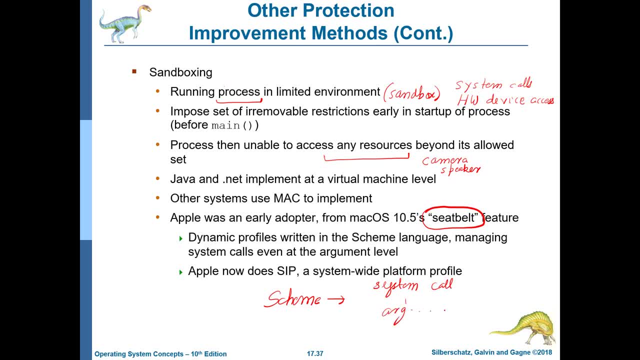 And by looking at these arguments of the system call, you can say that, look, these arguments are allowed in the sense that so what is a system call? It is asking some service from the kernel. So these are the services that are allowed and these are the services that are disallowed. 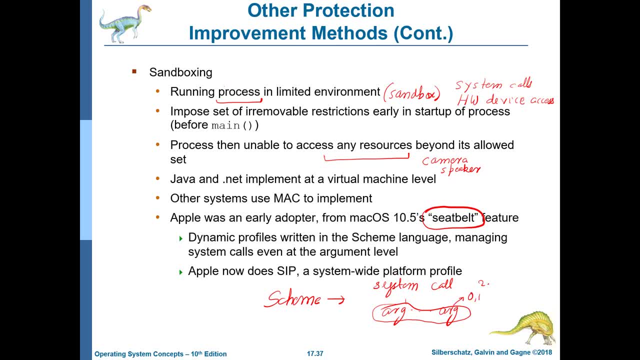 So, for example, if this argument is 0 and 1, I have no issue with it, but 2 and 3 I will not allow. So the seatbelt feature further gives the security subsystem much more control over what the application is doing. 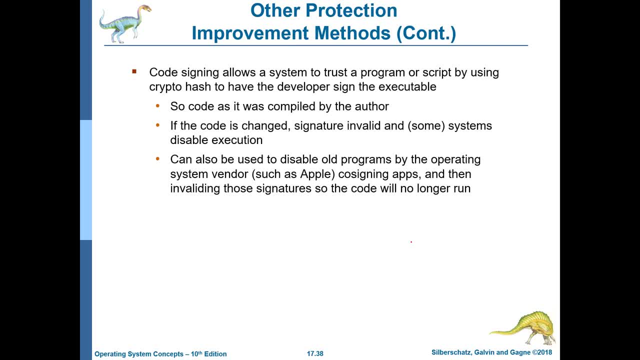 So we have already discussed code signing. So code signing basically verifies that it has been genuinely created by an author And furthermore it can also be used to kind of invalidate old programs which are either unsigned or were signed with a different signature. 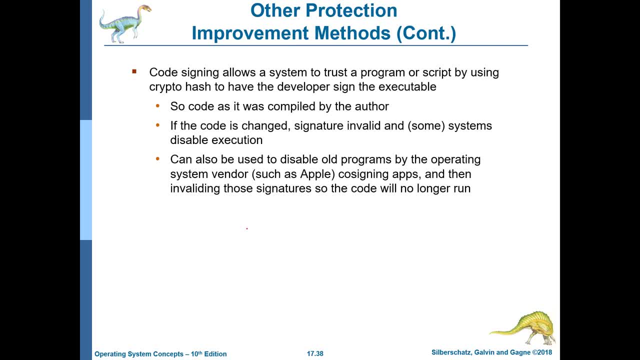 Because we are essentially invalidating those signatures. So code signatures is a common way of enforcing the authenticity of the code as well as the integrity of the code, And the integrity is basically sent by, like sending a MAC right, go back to the security. 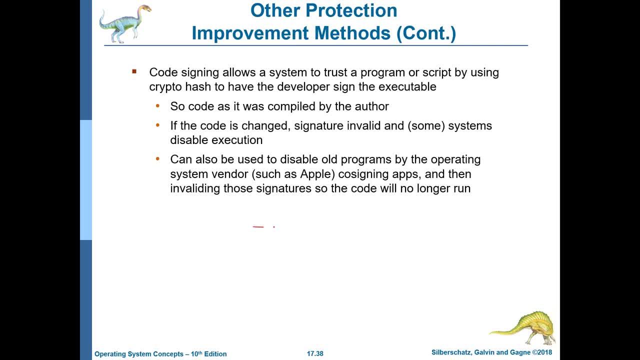 chapter, pretty much like sending a MAC along with the code. So this ensures that number 1, the code is authentic and number 2, it has not been tampered with. So then the client system can happily execute the code. 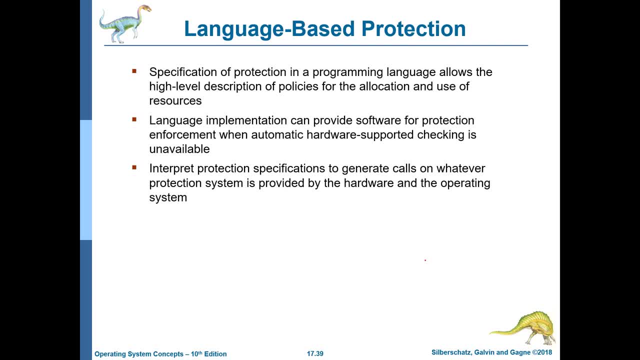 Then we can have language-based protection, So we can specify in a high-level language what are all the policies of the OS that we can, that we are going to allow and that we are going to disallow. So we have already discussed an example of this with the seatbelt feature, where basically 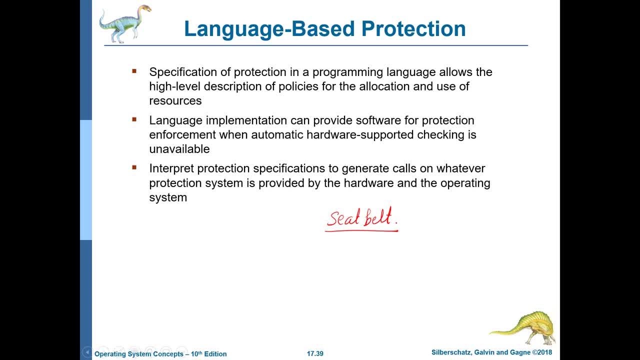 we have. We have checks at the high-level language level for the arguments of system calls. So this can be extended slightly more in the sense we can have checks for the code or we can have checks for specific instructions that are sent to sensitive hardware. 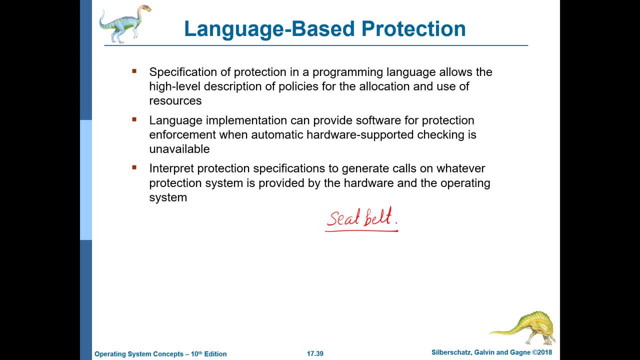 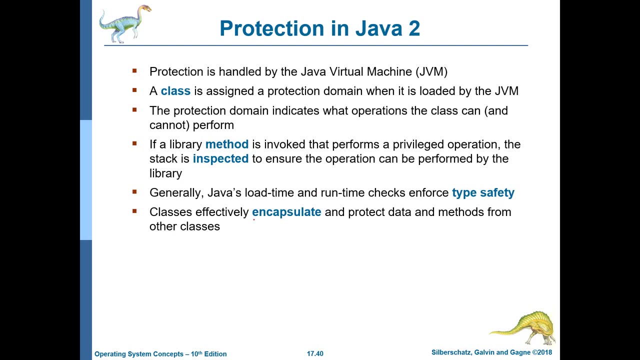 So of course there is a lot of space over here. In addition, we can have checks over network connections and network packets, So all of this would fall broadly in the domain of language-based protection. So coming to Java, So Java is a rather interesting language. 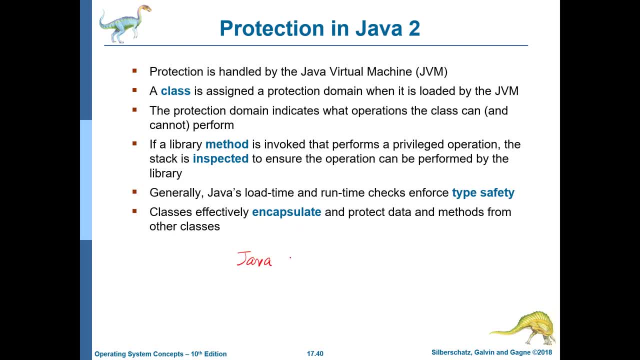 The reason being that what we actually run in Java is basically byte code. Byte code is written in a virtual ISA And while we and when we run the code, the byte code is actually runtime compiled. It is called just-in-time compilation, which means compiling just at runtime. 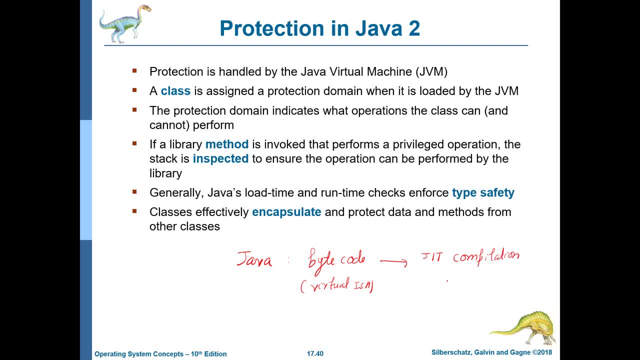 So the just-in-time compilation. what that is going to do is It is going to convert this to x86 code, If running on an x86 machine, that is, it is going to convert it to x86 instructions, And when it converts it to x86 instructions, it executes. 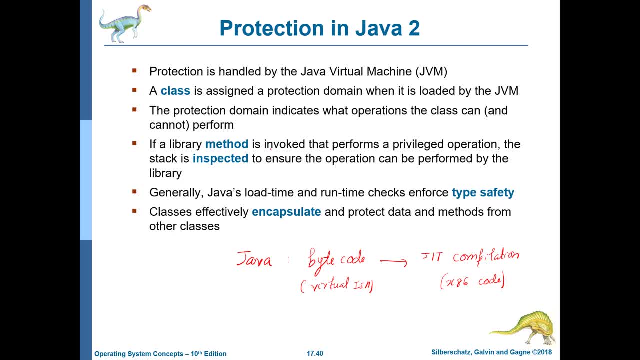 So during this process, every method can be scrutinized or inspected to see if it is performing a privileged operation and is that operation safe or not, And, furthermore, the stack of arguments can also be inspected At this time as a part of the compilation process, to check for safety. 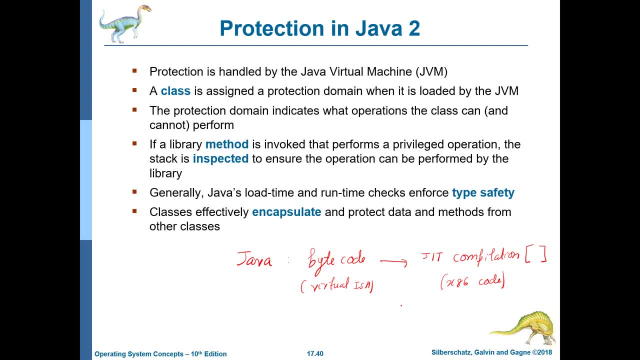 Furthermore, Java does allow type safety in the sense. C will happily allow you to typecast in a take, a float and kind of typecast into an int in an unsafe manner. But Java will not allow all of these because pretty much what happens is that Java wants. 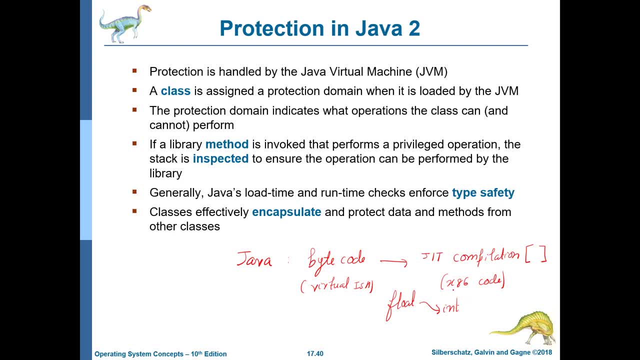 to stop you from using pointers. Otherwise, what will happen is that you can access any memory location. Consequently, in Java, pointers are not allowed. well, pointers are there in the sense that every object is actually represented by its pointer, But user processes are not allowed to manipulate those pointers. 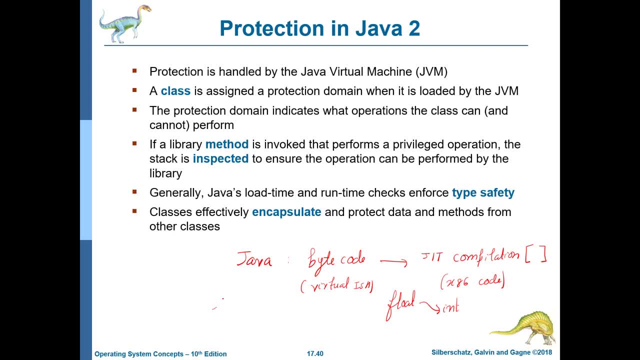 And this is where the safety comes from, because if you do not have pointers, you cannot access arbitrary memory locations and basically create havoc by reading or writing anything that you want. This is something that Java explicitly prohibits. And this is also where the notion of type safety comes in, because in C you can happily 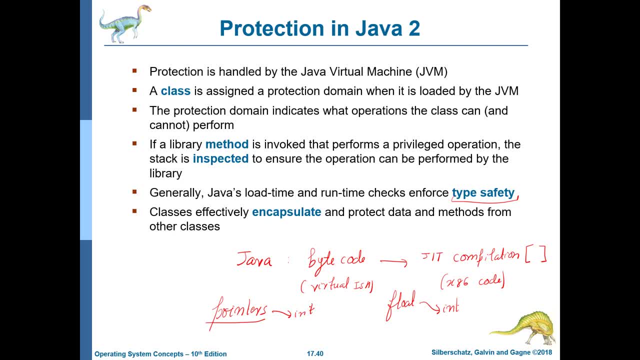 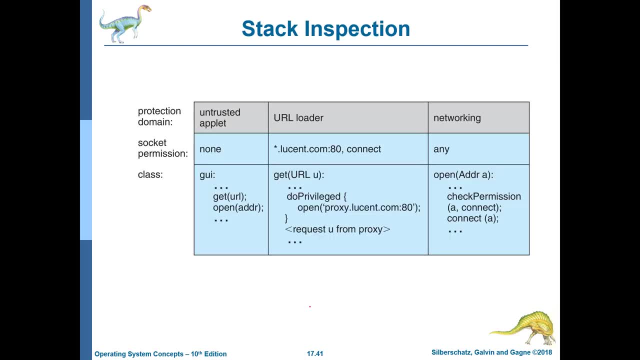 typecast a pointer to an integer and then do pointer arithmetic on it. This is not something that Java allows. Now, coming to the stack inspection. So Java does that in the sense that whenever we are opening, let us say, some remote network, 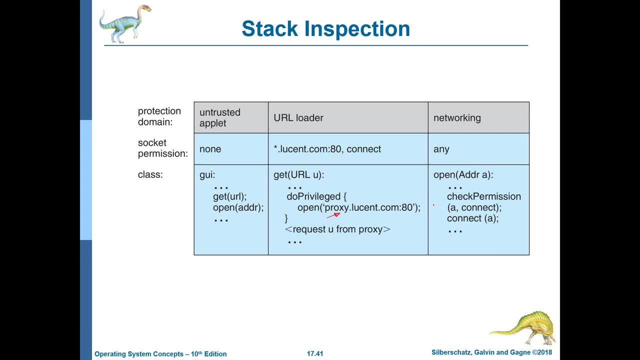 site, Let us say proxy network, Let us say proxylucentcom, and we are checking whether I have permissions to access that or not. All of these things the Java virtual machine can do very well because it basically has access to all the runtime code that the binary is executing.